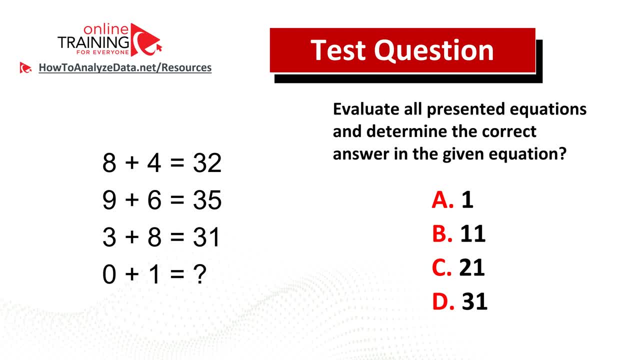 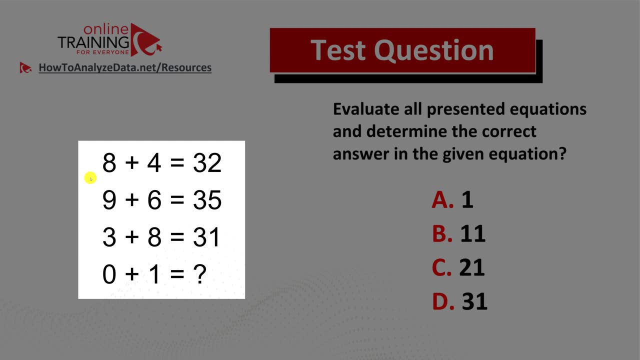 Now might be a good time to pause this video to see if you can come up with the answer on your own. Did you come up with the answer? Let's continue to see how we can solve this challenge and get to the solution together. Before we jump to the solution, let me give you some tips. It is still a decimal system that we're 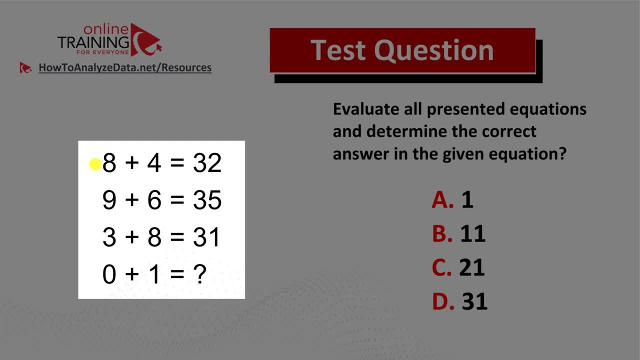 dealing with here, And if we continue with this assumption, we can see that the sum of numbers in all cases is a little bit higher than the actual numbers in the decimal system. 8 plus 4 in reality is 12,, not 32.. But the difference between 32 and 12 is 20.. Hopefully this gives. 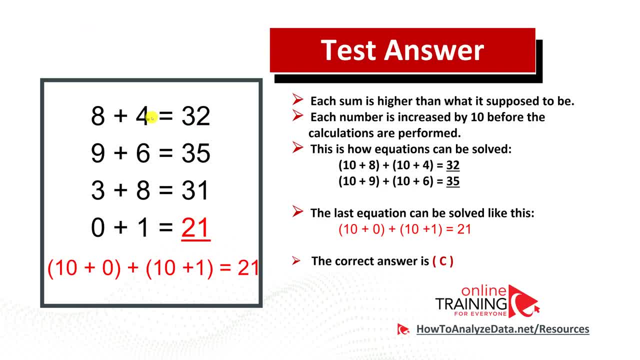 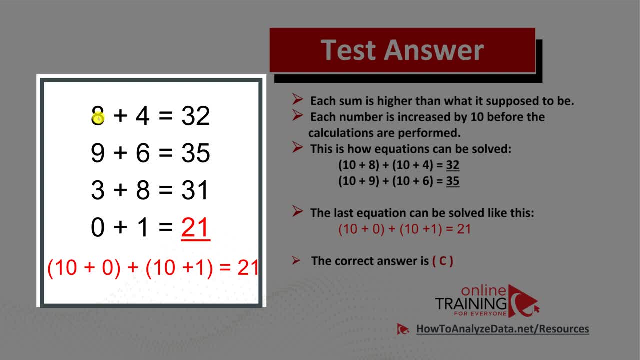 you some tip Now, continuing with this logic, Basically, what's happening is that each number is incremented by 10 before the calculations are performed. For example, 8 plus 10 is 18 and 4 plus 10 is 14.. 18 plus 14 equals 32.. Same calculations. 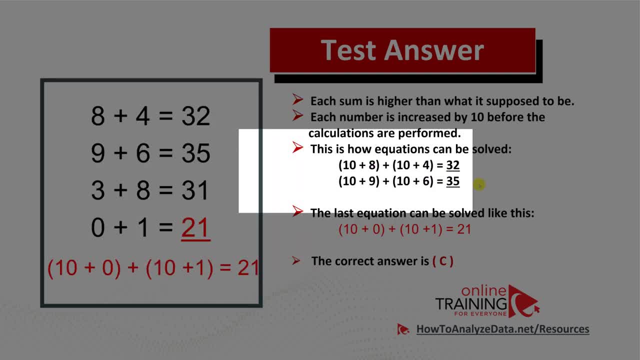 are done with the second, third and fourth equations. For example, 19 plus 16 equals 35. And the last equation can be solved like this: 10 plus 0,, 10 plus 1, equals 10 plus 11, equals 21.. So the correct choice here is choice C 21.. Hopefully by now. 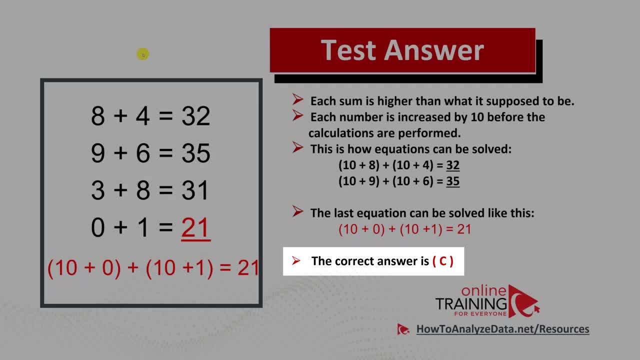 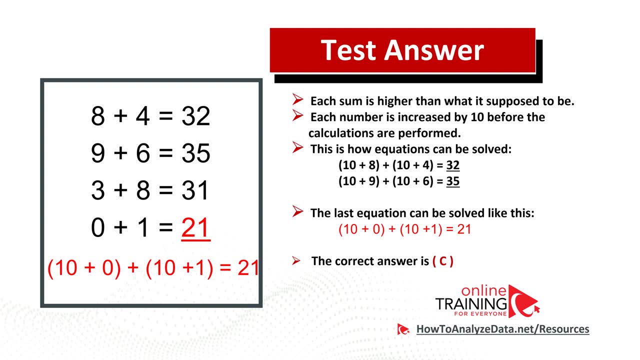 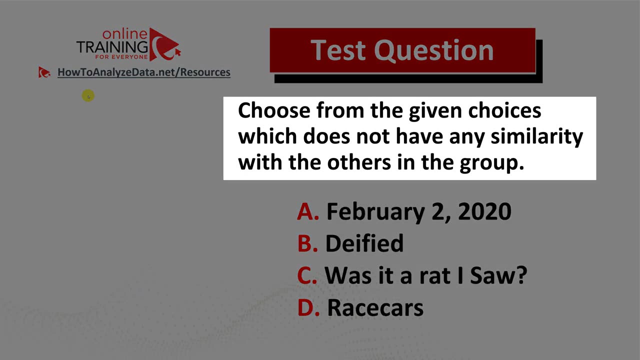 you know how to answer these types of questions in the test. But in case you need more questions or practice problems, please make sure to check out my aptitude test ebook in the description section of this video. And now here's the question for you to try. Please choose from the given. 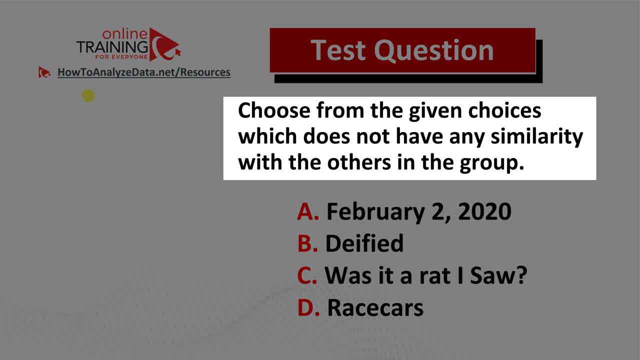 choices and identify which item does not have any similarity to the answer And, if you do choose, which option is your favourite. But if you do choose one of these, Question 1. Which of the following options does the two options offer similarity? 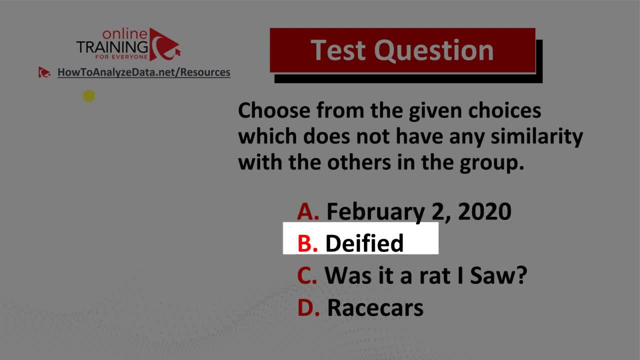 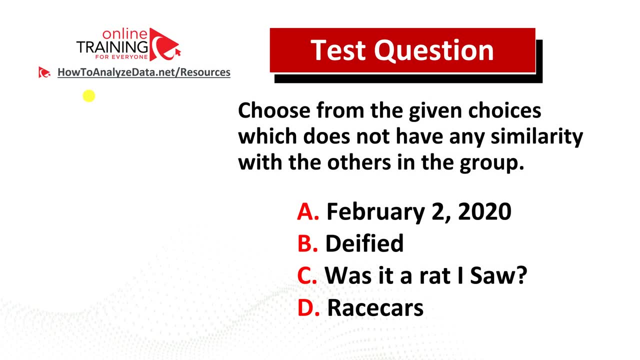 with the others in the group And you have 4 different choices. February 2, 2020.. Day 5. Was it a rat? I saw Race cars. Do you think you know the answer? Feel free to pause this video and try to solve it. 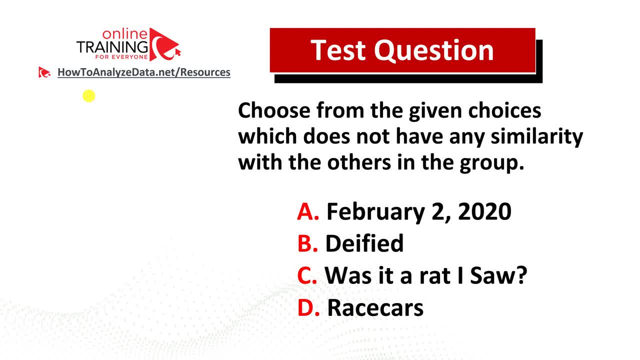 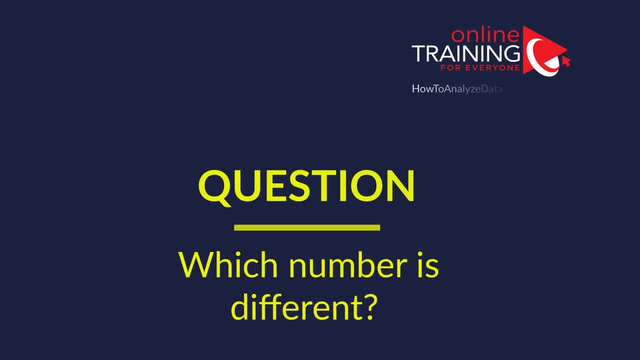 And if you came up with the answer, feel free to post it in the comment section of this video so I can give you my feedback. Thanks for participating. Let's look at the interesting and tricky question, Question 2.. Who is more likely to die? 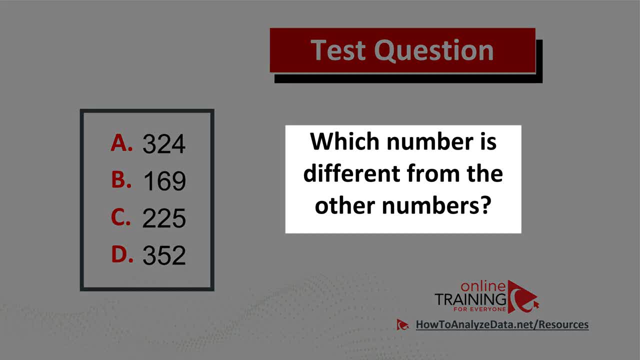 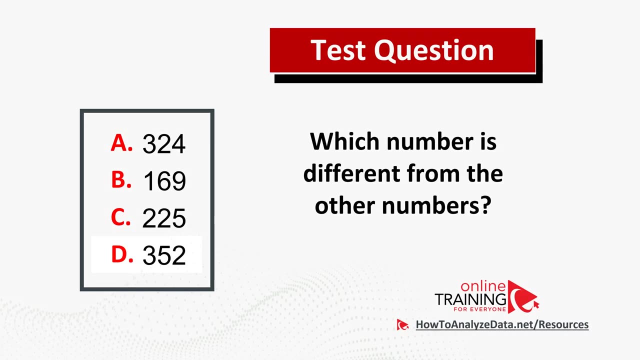 frequently see on the test Which number is different from the other numbers And you have four different choices: Choice A: 324.. Choice B: 169.. Choice C: 225.. And choice D: 352.. Do you think you know the answer? Now might be a good time for you to pause the video to see. 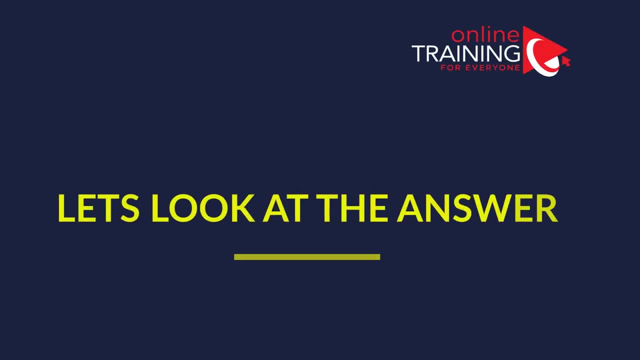 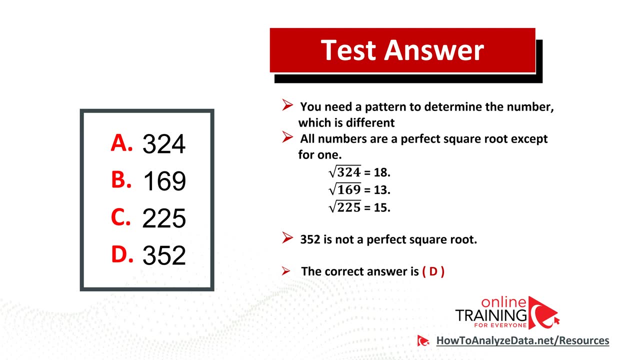 if you can come up with the answer on your own. Did you come up with the answer? Let's see if we can get to the solution together. As usual, to get to the answer, you need to determine the pattern and understand which three numbers match the pattern and which one number does not belong. 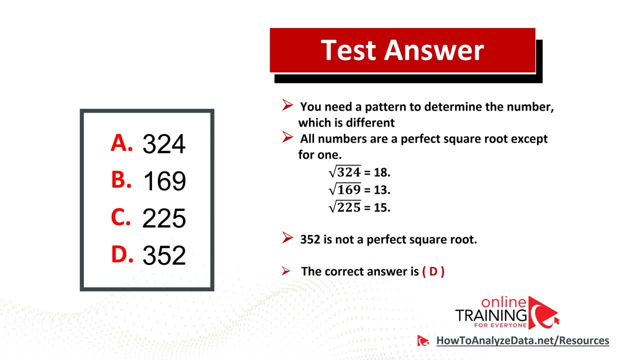 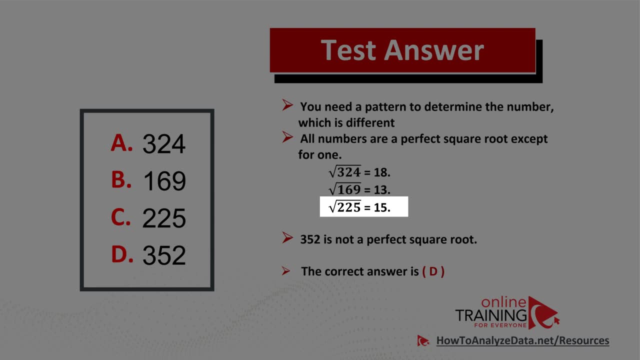 to the pattern. In this case, the pattern is square root. All numbers here. you can see that three numbers listed here are a perfect square root. A square root of 324 is 18.. A square root of 169 is 13.. And square root of 225 is 13.. And square root of 225 is 13.. And square root of 225. 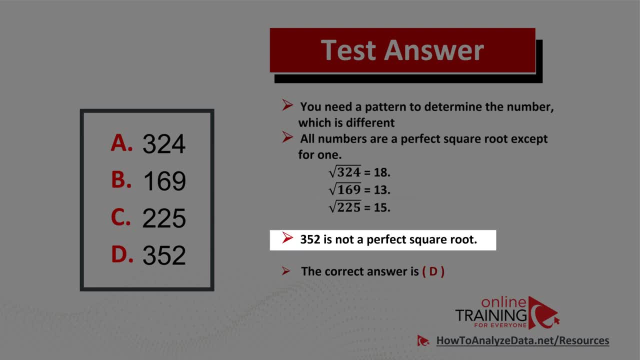 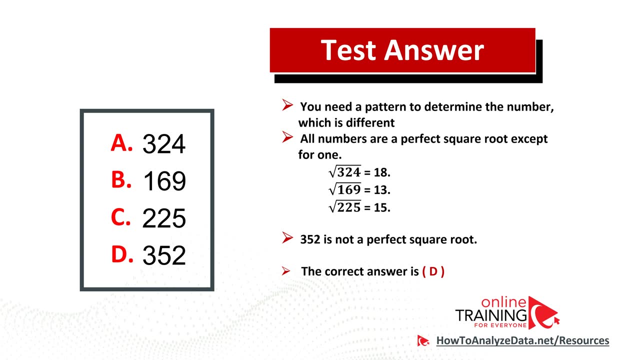 is 15.. In this case, 352 is not a perfect square root, So the correct answer here is choice D 352.. Hopefully you've nailed this question, But in case you need to practice more, please make sure to check out my ebook in the description section of this video. 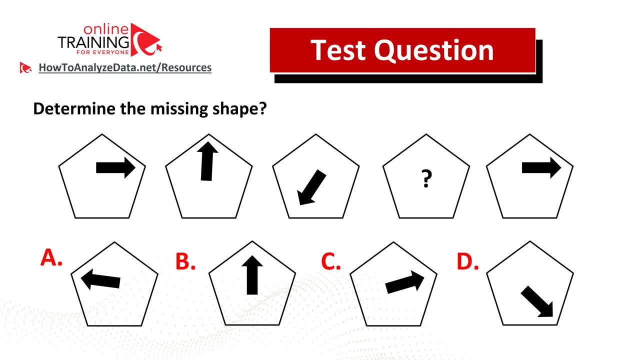 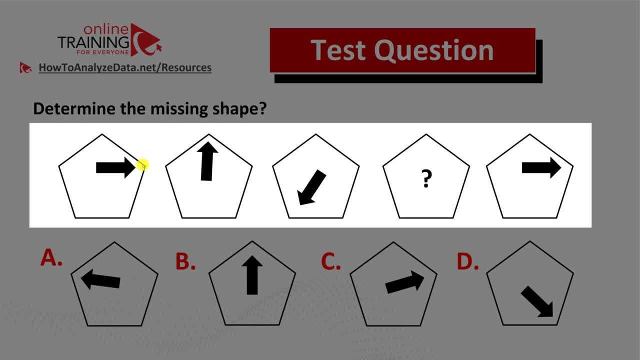 Let's look at the interesting and tricky question we frequently see on the test: Determine the missing shape. You're presented with the sequence of five shapes. All of them are pentagons And in each one arrow points in a different direction. There are three shapes with arrow. The fourth shape, 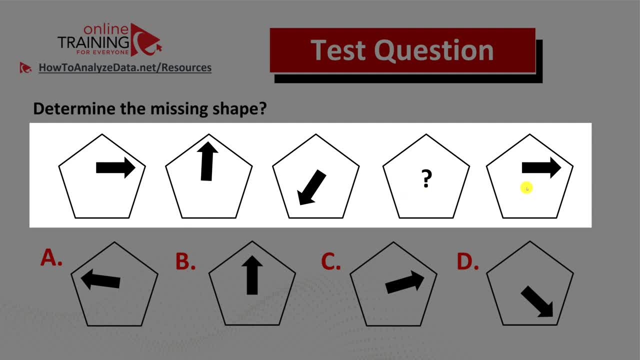 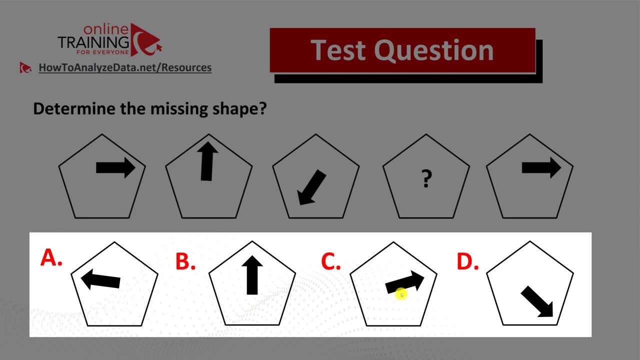 has a missing arrow, And this is what you need to determine. And then there's also a fifth shape And you have four different choices. All of them contain pentagons with arrow pointing in a different direction. Do you think you know the answer? Now might be the good time to pause this. 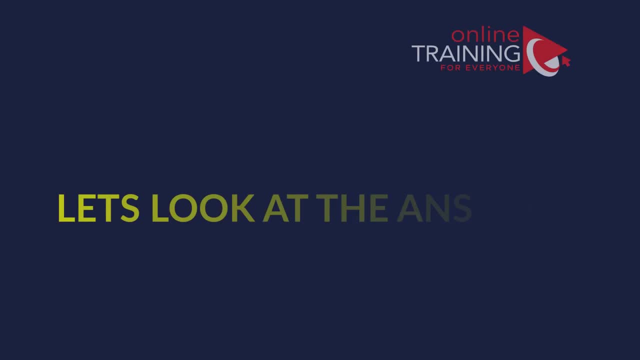 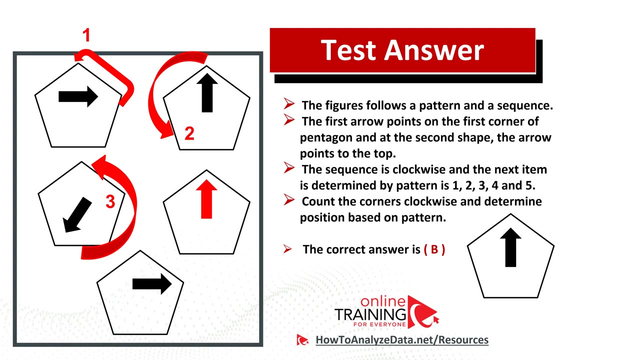 video to see if you can come up with the answer on your own. Did you come up with the answer? Let's see if we can solve this challenge together. To solve pattern questions, you need to determine the sequence in the pattern And in this particular one we have a sequence of items moving counterclockwise To determine. 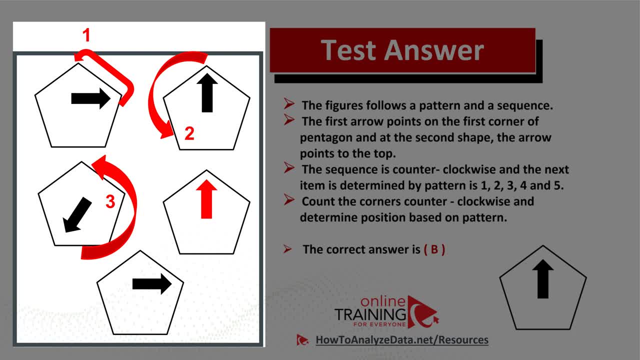 the position of the next arrow. we need to determine the pattern. As you can see, the position of the arrow in the next one is not straight figure, is determined by the sequence number. For example, in the item 1 arrow points to one o'clock, to the first angle of the pentagon. For the second position. 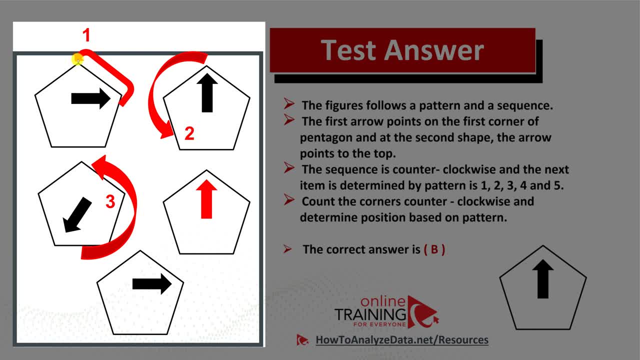 you need to move counterclockwise and move it into the next corner. For the next one you need to move two steps, because the sequence would be two, because this is the second shape. and once you move to the second shape, you move to the eight o'clock in the eight o'clock corner of the pentagon, As you. 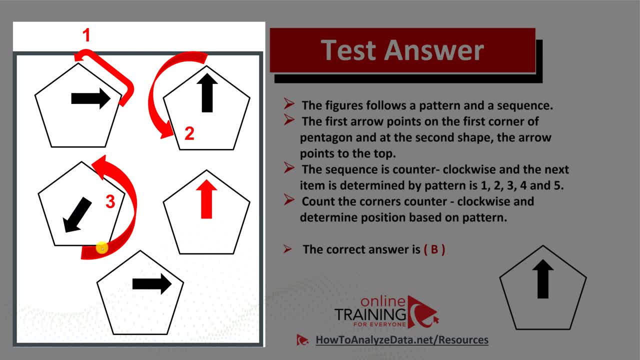 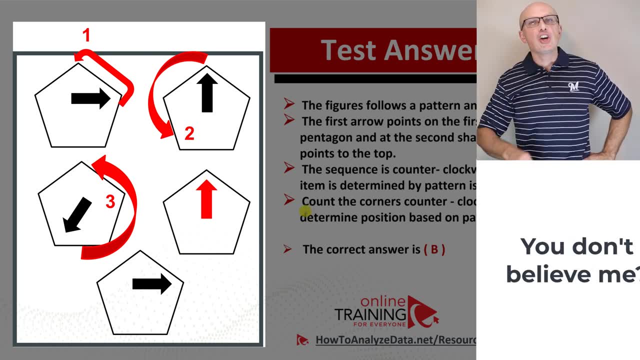 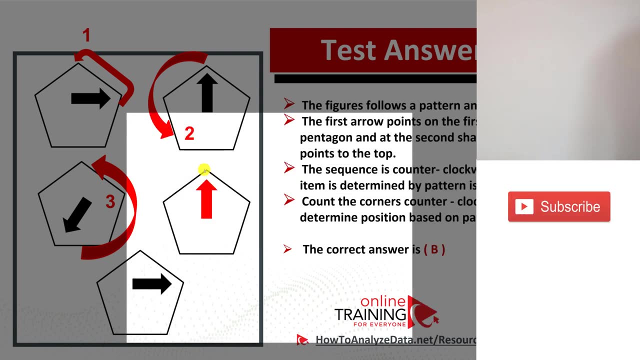 continue moving, your next move would be jumped through three corners of the pentagon and you will be at twelve o'clock, and this is the position of the arrow we're trying to determine. So the correct answer here is choice B, pointing at twelve o'clock. and if we continue the sequence, just to verify, to make sure we 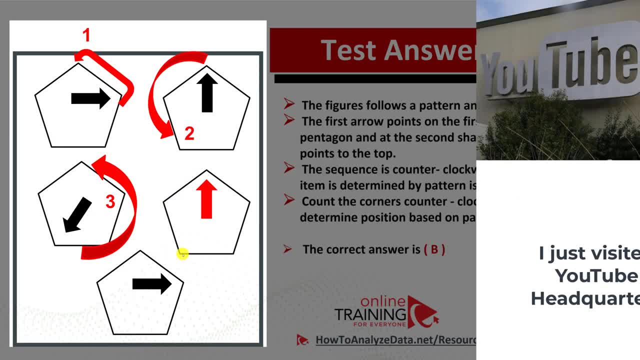 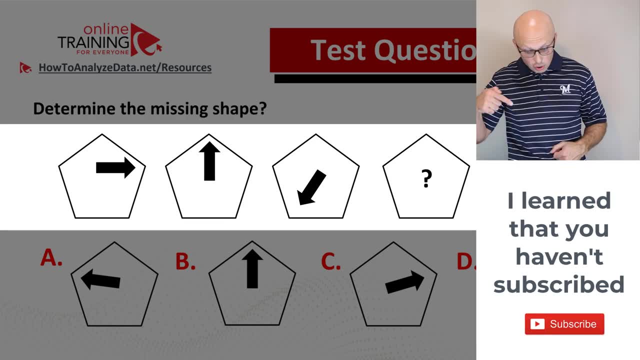 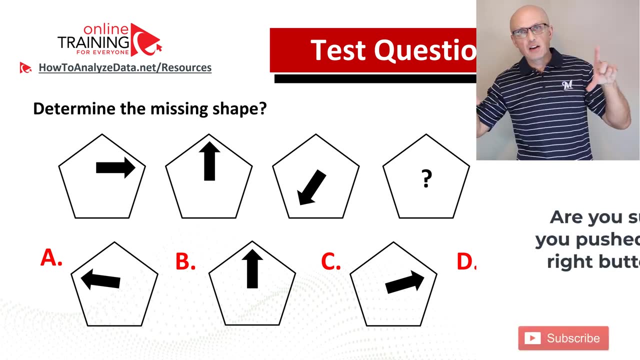 did it correctly, we can add four: one, two, three, four, which points us back to one o'clock, which is item number five, represented in the original question. Hopefully you've nailed this question and maybe even figured it out, and I hope that my instructions give you ability to answer these types of questions in the 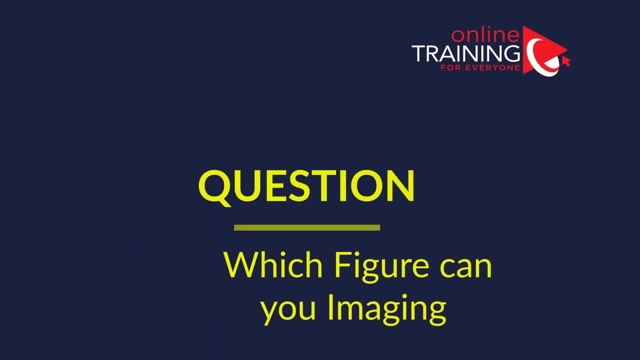 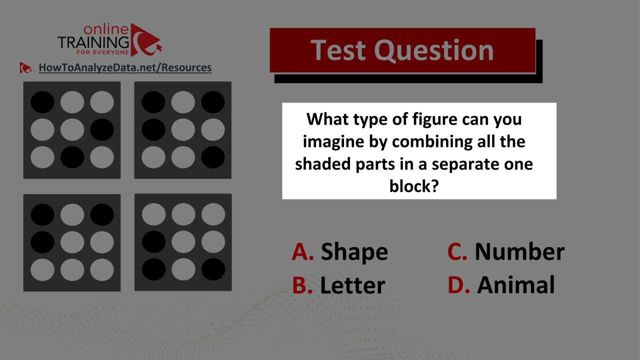 test. Here's the tricky question from the real test: What type of figure can you imagine by combining all the shaded parts in a separate one block and your four choices Shape, letter, number or animal? Do you think you know the answer Now? 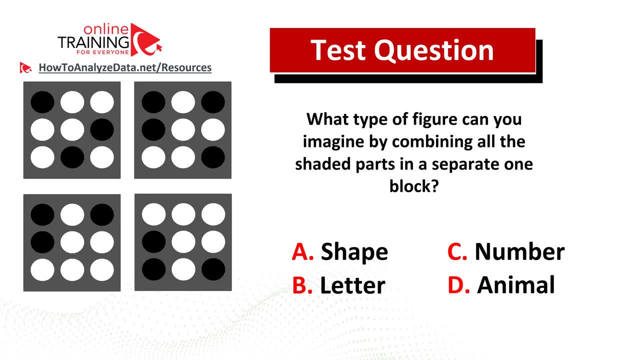 might be a good time to pause this video to see if you can come up with the answer on your own. Did you come up with the answer? Let's see how we can solve this challenge and get to the solution together. The tricky part here is combining all four blocks. 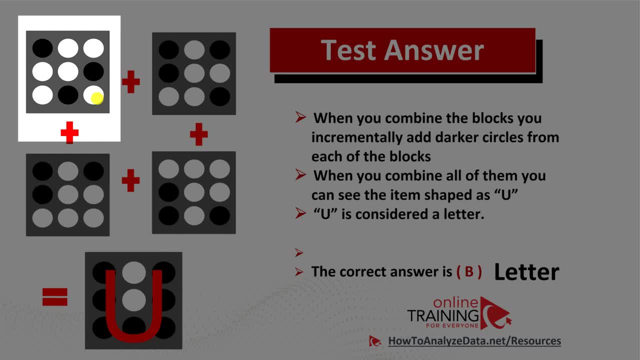 right in your memory and using your imagination to come up with the final answer. But when you combine the blocks incrementally, you add darker circles into one single image and final image here in the sequence, represents all darker circles added in one image And, as you can see, 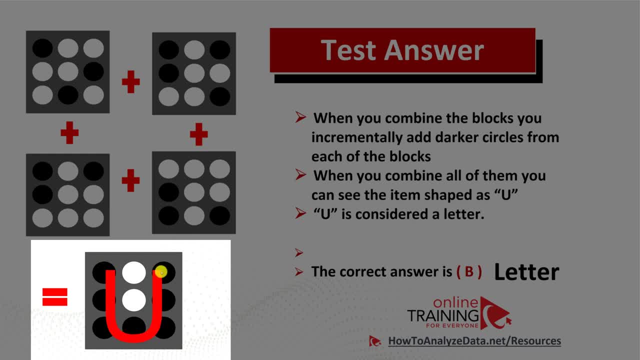 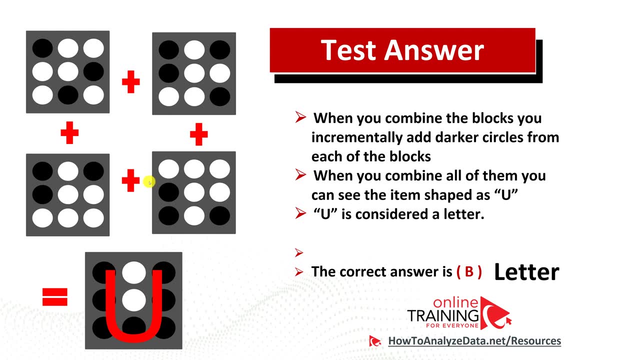 the shape of the darker circles represent letter U, so the correct answer here is choice B letter. Hopefully you've nailed this question and now know how to answer these types of questions in the test, But in case you need more questions or practice problems, please make sure to check out my aptitude. 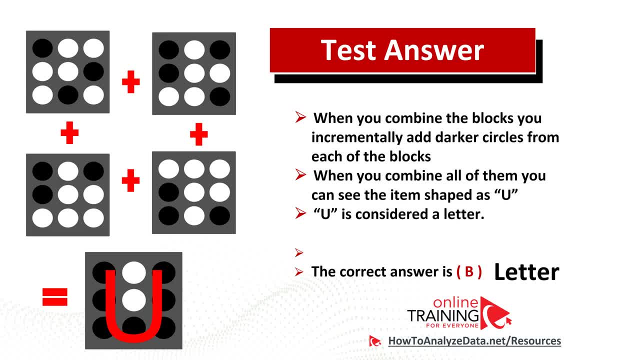 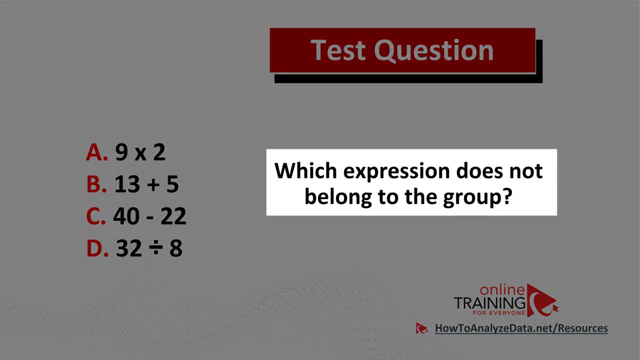 test ebook in the description section of this video. And now here's the question for you to try: Which expression does not belong to the group? And you have four different choices: 9 by 2,, 13 plus 5,, 40 minus 22, or 32 divided by 8.. Do you think? 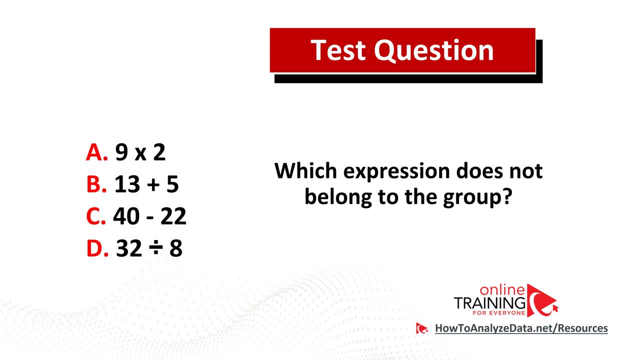 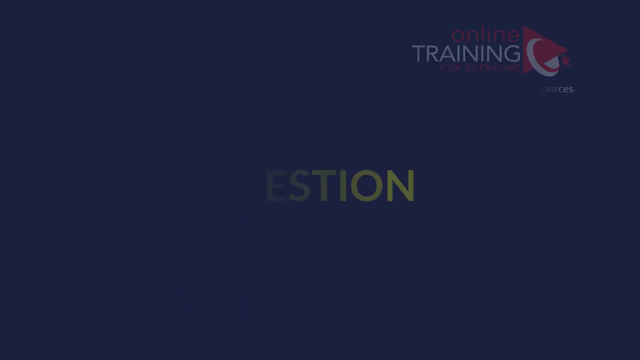 you know the answer, Feel free to pause this video and try to solve it, And if you came up with the answer, feel free to post it in the comment section of this video and I'll give you my feedback. Thanks for participating. Some of you might find this question tricky, but regardless of whether you can, 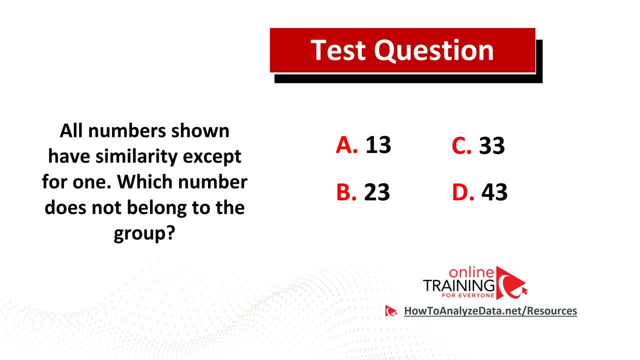 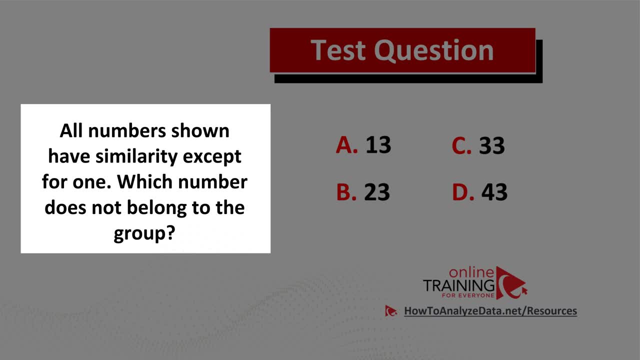 solve it or not on your own. you will be excited to learn the solution to this real-life assessment test question. All numbers shown have similarity except for one, Which number does not belong to the group, And you have four different choices: Choice A 13,, choice B 23,, choice C: 33, and. 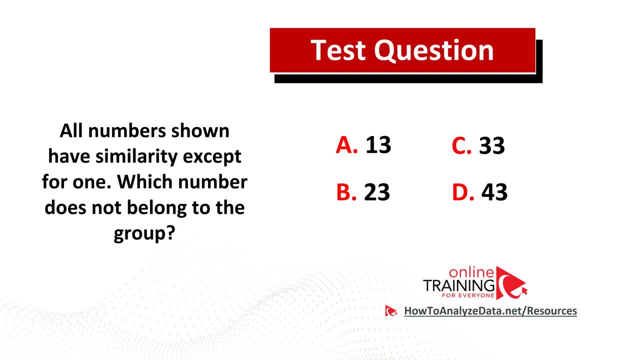 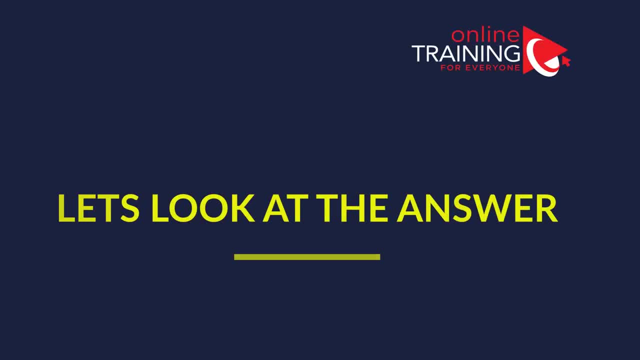 année 43.. Do you think you know the answer? Now might be a good time to pause this video to see if you can come up with the answer on your own. Did you come up with the answer? Let's continue to see how we can solve this. 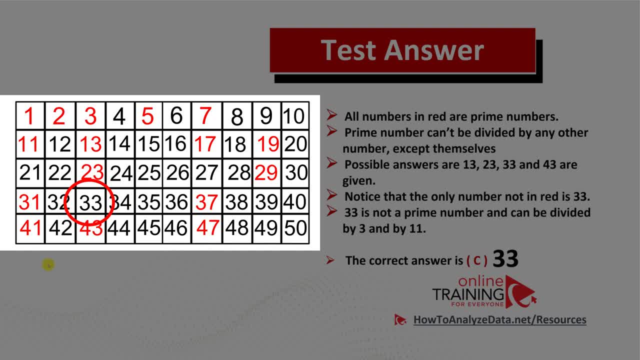 challenge together. The solution lies in understanding very simple math concept, the concept of prime numbers. You see on the left the grid of numbers from 1 to 50. And all the numbers that are considered prime numbers are highlighted by 1. in red. What is prime number? Prime number is the number that you can only divide by itself. 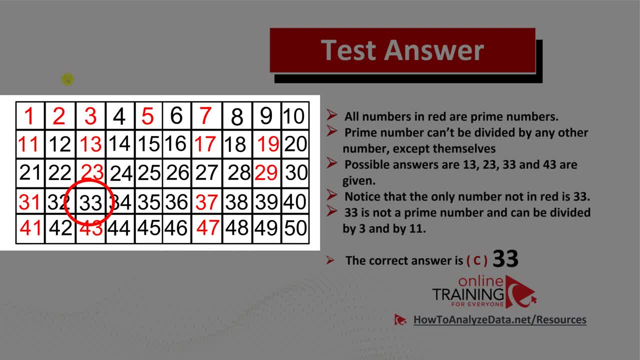 You cannot divide it by any other number, For example 1. you cannot divide by anything but 1.. Same for 2,, 3,, 5,, 7, and etc. Out of all the numbers presented in the question, 33 is not a. 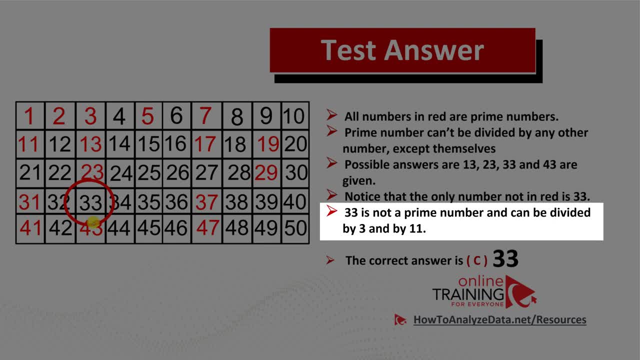 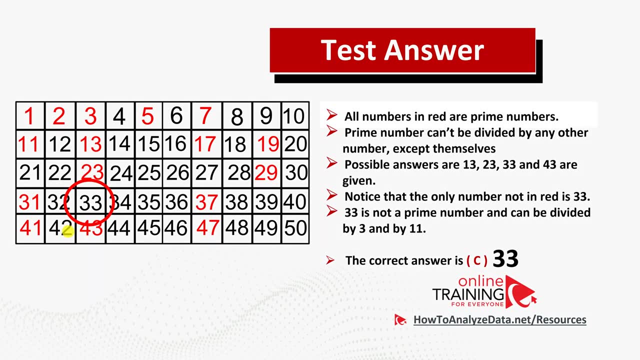 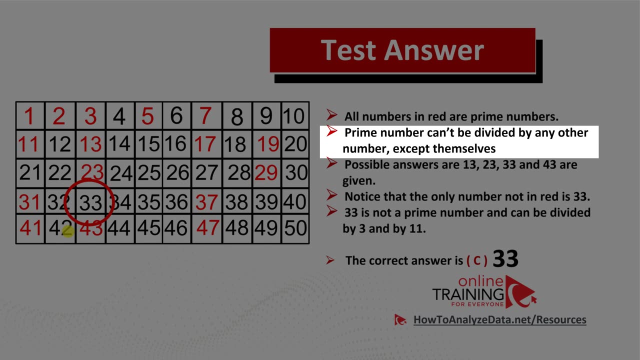 prime number because 33 can be divided by 3 and also can be divided by 11.. So the correct answer here is choice C 33.. Let's recap: All numbers in red presented in the grid are prime numbers. Prime number cannot be divided by any other number except themselves. Possible answers are 13,, 23,. 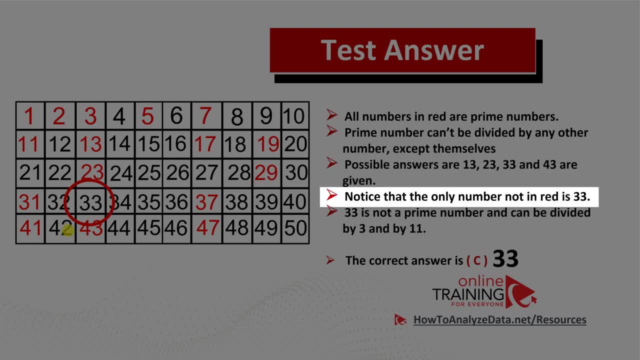 33, and 43. And the only number that is not a prime number is 33.. 33 is not a prime number because it can be easily divided by 3 and by 11. So the correct choice here is choice C 33.. 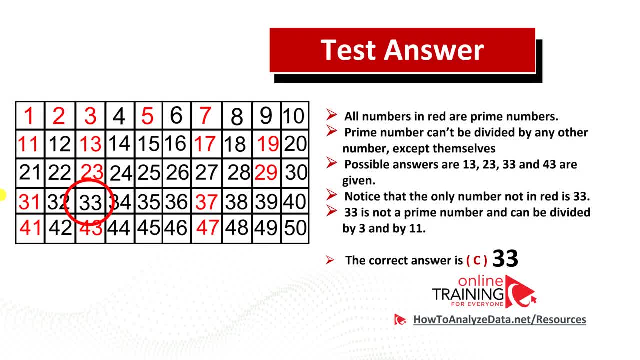 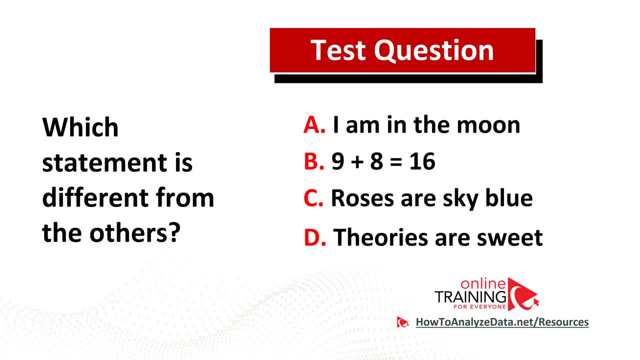 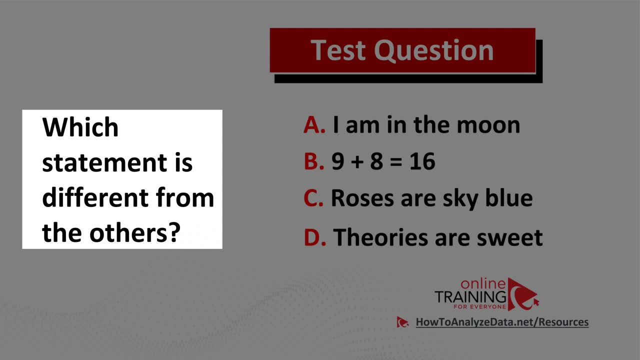 Hopefully you've nailed this question and now know how to answer these types of questions on the test. And now here's the question for you to try. Please make sure to post your answer in the comment section of this video so I can give you my feedback. Which statement is different from? 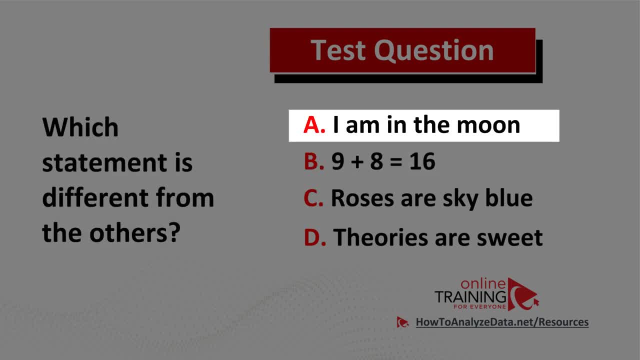 the others. The first statement, A- I'm in the moon. Choice B: 9 plus 8 equals 16.. Choice C: roses are sky blue And D- theories are sweet. Do you think you know the answer? Feel free to pause this video and try to solve it. 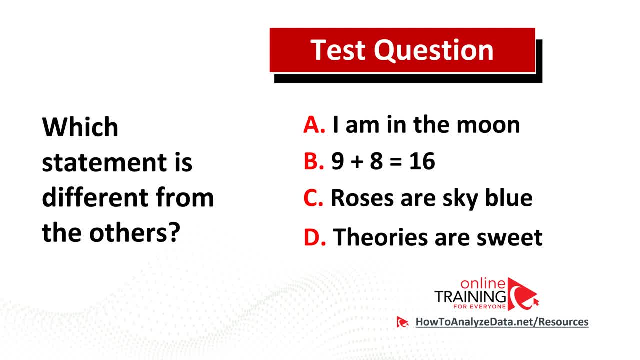 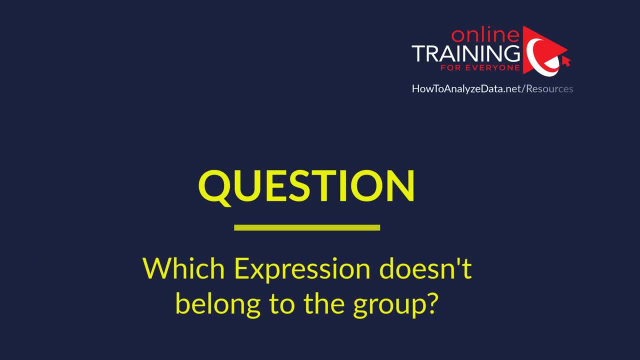 And if you came up with the answer, feel free to post it in the comment section of this video so I can give you my feedback. Thanks for participating. One comment is: roses can be blue. Please search on Google blue roses and you will see the picture. Are you ready for this challenging problem? Let's. 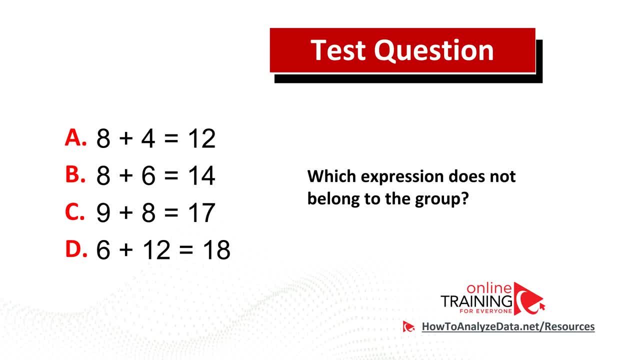 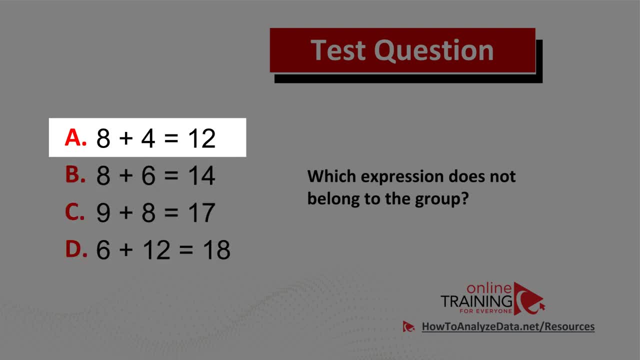 look at the very interesting and tricky question you might frequently see on the test Which expression does not belong to the group? And you have four different expressions: Choice A: 8 plus 4 equals 12.. Choice B: 8 plus 6 equals 14.. Choice C: 9 plus 8 equals 17.. And 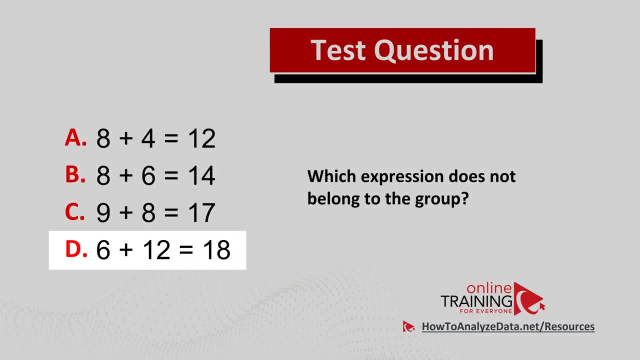 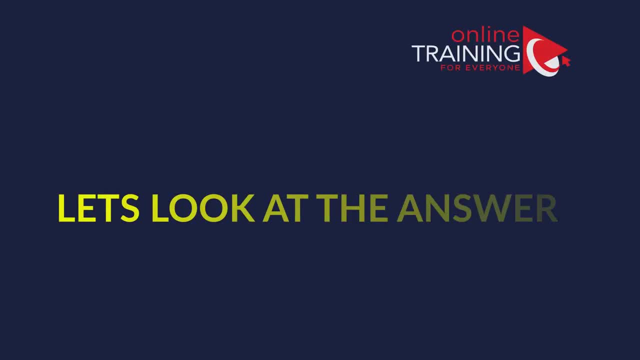 choice D: 6 plus 12 equals 18.. Do you think you know the answer? Now might be the right time for you to pause the video to see if you can come up with the answer on your own. Do you think you know? 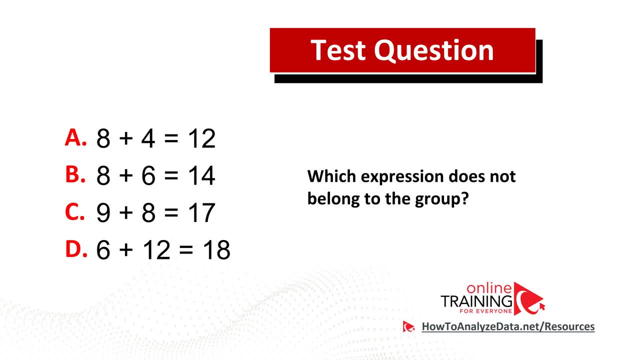 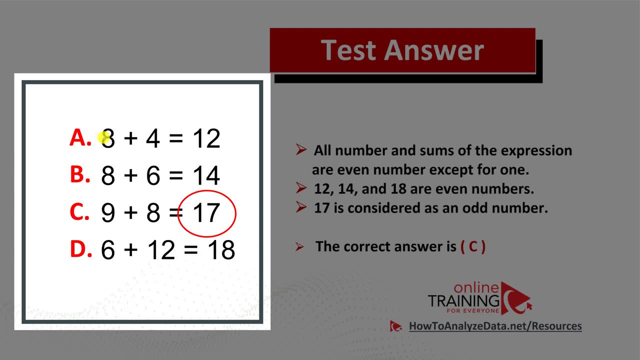 the answer. Let's continue to see if we can solve this question And if you can, please do so. Let's continue to see if we can solve this challenge together. What's interesting about this question is the fact that we're dealing here with odd versus even numbers. You see that. 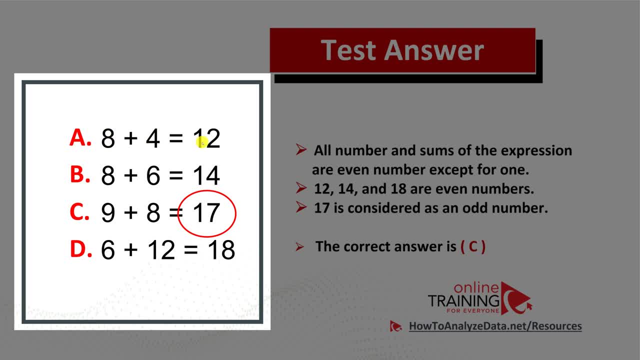 expression A has all the even numbers: 8 and 4 equals 12.. Expression B is the same thing: 8 plus 6 is 14, all even numbers, Same with expression D: 6 plus 12 equals 18.. So the 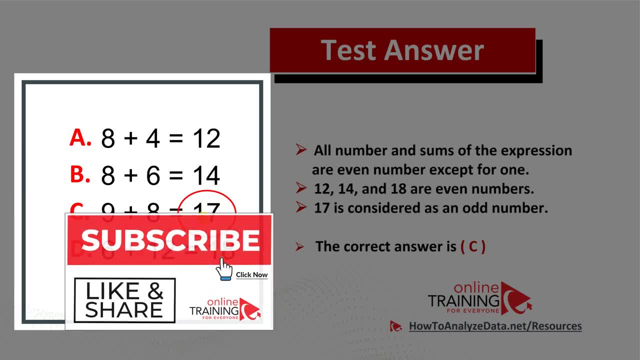 expression C has two odd numbers, 9 and 17.. And if you look at the answers, you can also figure it out by looking at the answer. The answers are 12,, 14, and 18 for solutions A, B and D And for the. 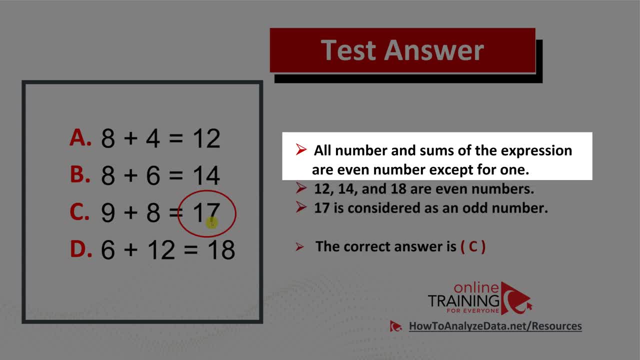 C, the answer is 17.. So let's recap: All numbers and sums of the expression are even numbers, with the exception of one: 12,, 14, and 18 are even numbers, but 17 is the odd number, So the correct. 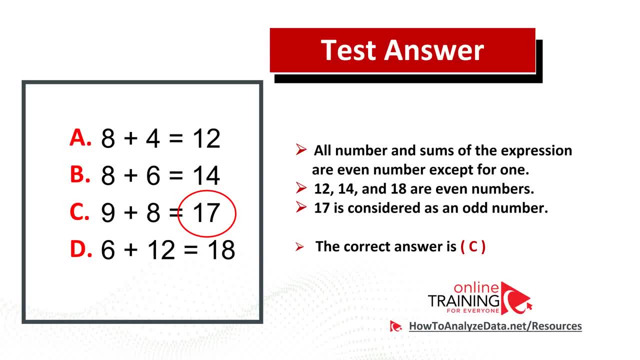 answer here is choice C 17.. Hopefully you've nailed this question and got to the correct answer on your own, But in case you need more questions or practice problems, please make sure to check out the description of this video for my aptitude test questions. PDF ebook. 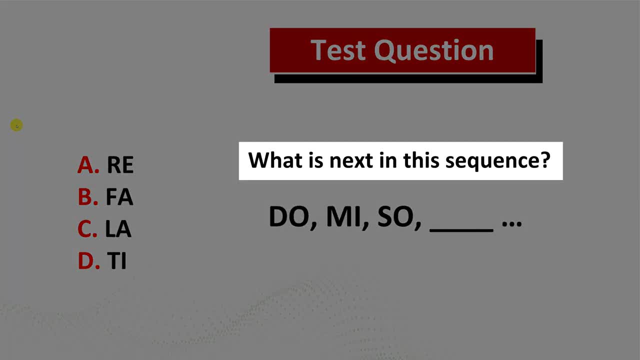 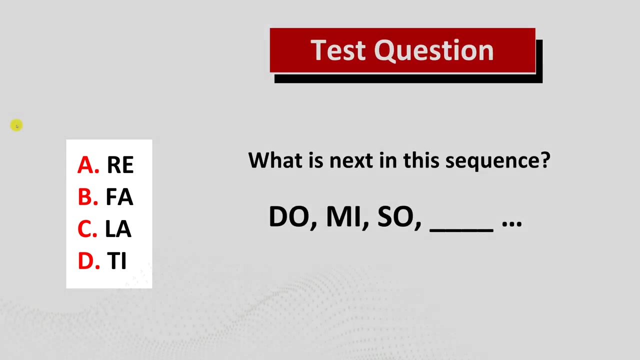 And now here's the question for you to try: What is the next item in the sequence? And you have series of items, Do me so. and then the next item that you need to determine, And you have four choices: Re fa la ti. Do you think you know the answer? Feel free to pause this video. 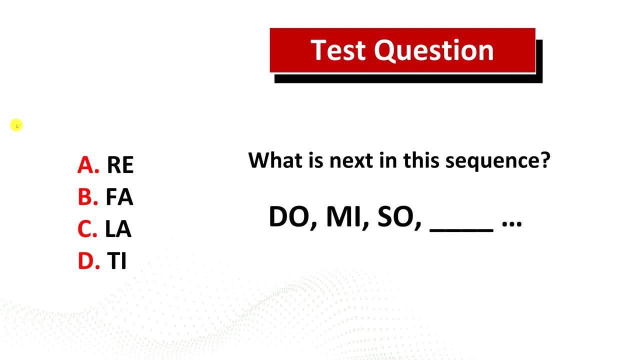 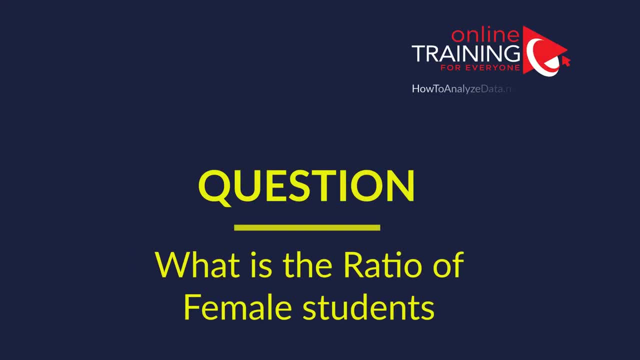 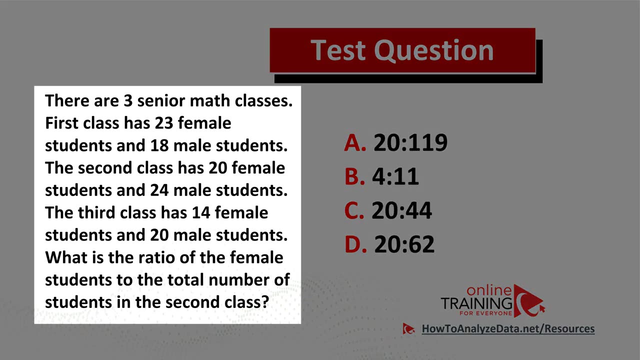 and try to solve it, And if you came up with the answer, feel free to post it in the comments. Let's look at the tricky question you might frequently see on the test. There are three senior math classes. First class has 23 female students and 18 male students. The second class 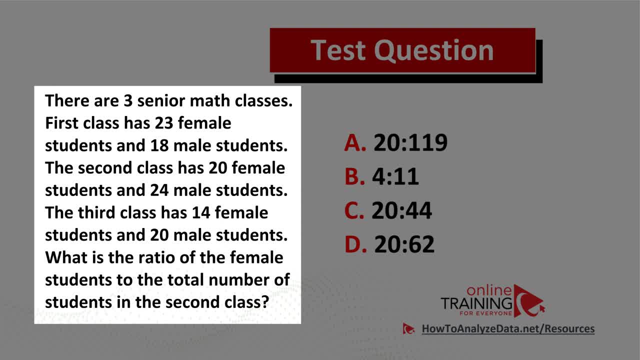 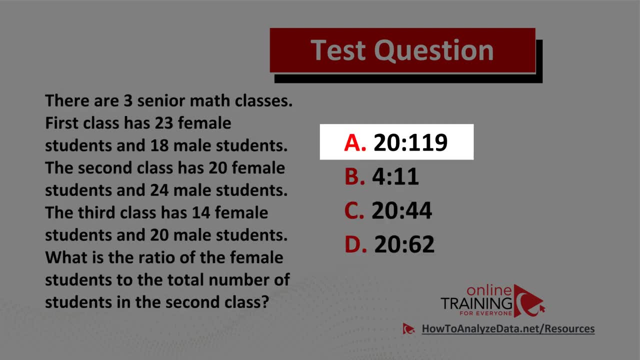 has 20 female students and 24 male students, And the third class has 14 female students and 20 male students. What is the ratio of female students to the total number of students in the second class? And you have four different choices: Choice A- the ratio 20 to 119.. Choice B- the ratio 4 to 11.. 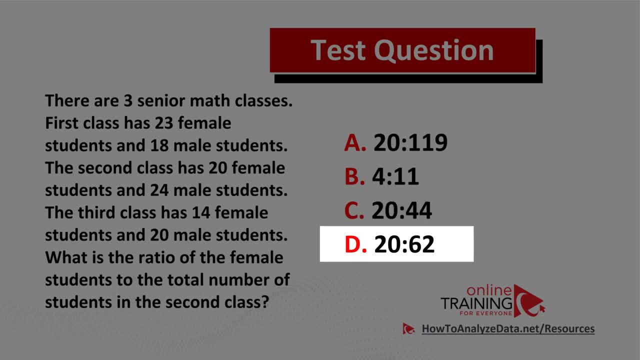 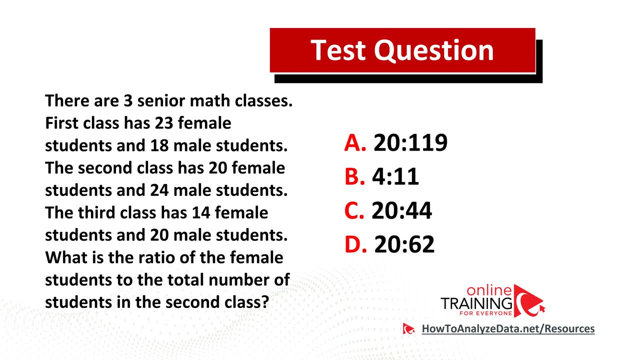 Choice C: 20 to 44. And choice D- 20 to 62.. Do you think you know the answer? Now might be a good time to pause this video to see if you can come up with the answer on your own. 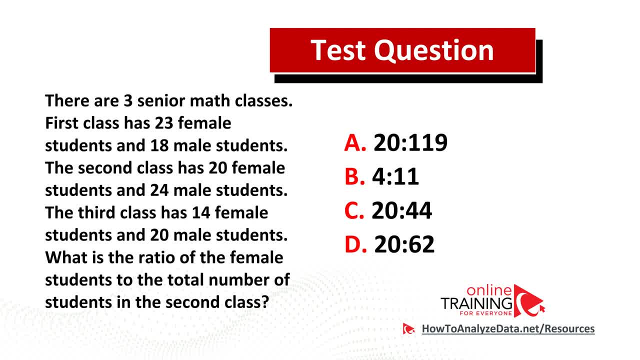 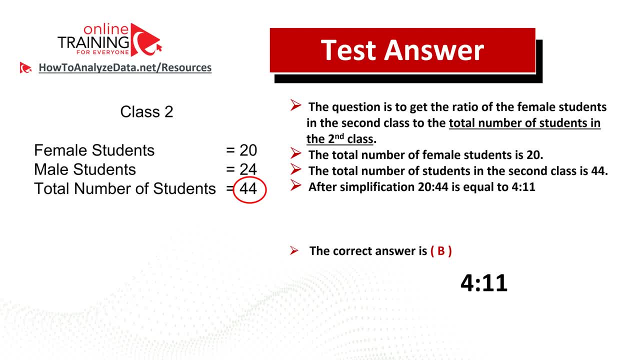 Did you come up with the answer. Let's continue to see if we can solve this challenge and get to the correct solution together. The tricky part here is that you're presented with lots of data about first, second and third classes, But the question only asks you about the ratio in the second class. 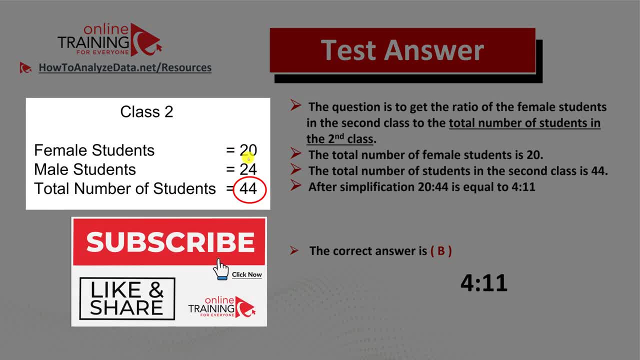 So the total number of female students in the second class is 20.. And total number of male students is 24, which is irrelevant already. Plus, you have data for the first and the third class, which is also irrelevant and not used in this class. 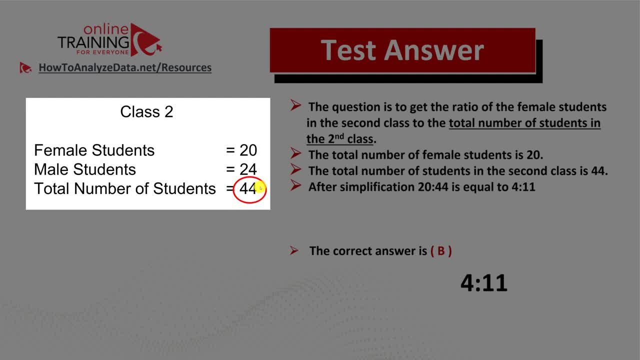 And the total number of students in the second class, which is another important piece of information, is 44. So the only two pieces that you would use is number of female students in the second class, which is 20, as well as the total number of students in the second class. 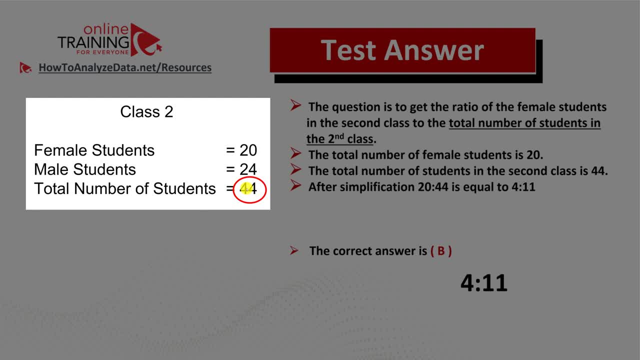 which is 44. So the ratio is 20 to 44, which, after simplification, leads you to 4 to 11 ratio. So the correct answer is choice B, 4 to 11.. Hopefully you've nailed this question. And now, 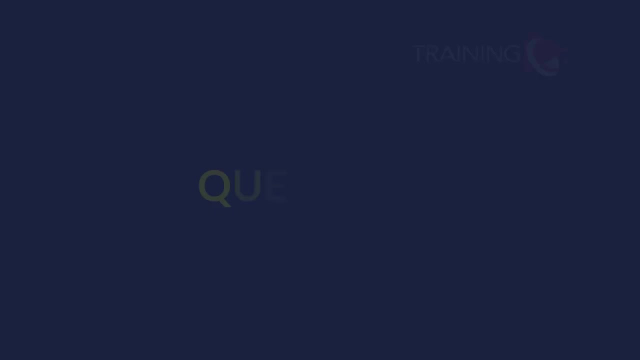 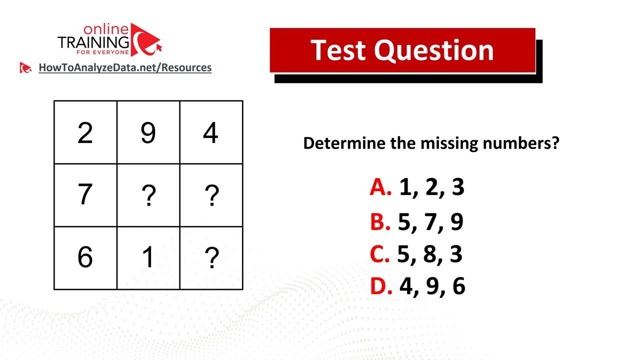 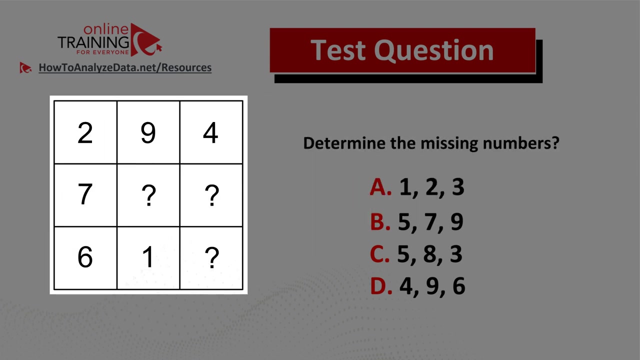 here's the tricky question from the real test, But somehow I have a feeling that you might come up with the answer: Determine the missing numbers And you have a square which has 9 numbers And 3 out of 9 numbers are missing And you have 4 different choices: Choice A, 1, 2, 3.. Choice B: 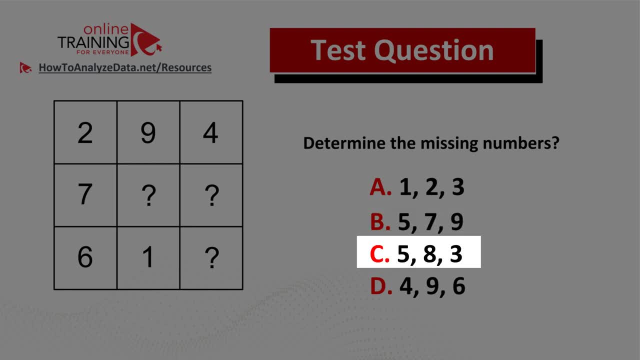 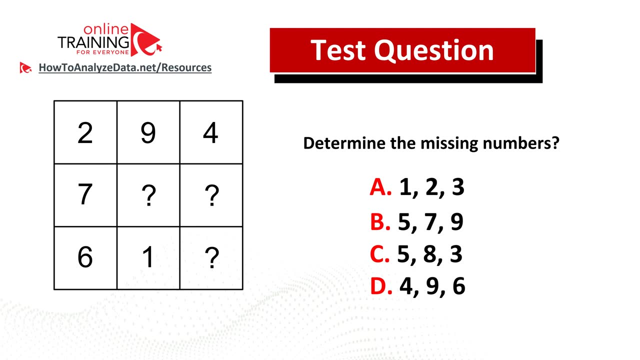 5, 7, 9.. Choice C: 5,, 8,, 9.. And you have 4 different choices: Choice A: 1, 2, 3.. Choice B: 3. And choice D: 4, 9, and 6.. Do you think you know the answer? Now might be the right time to. 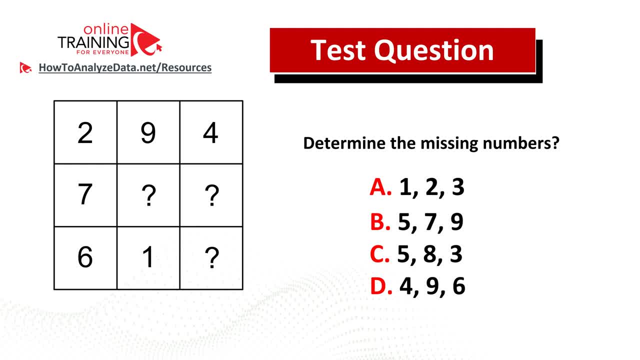 pause this video to see if you can come up with the answer on your own. Did you come up with the answer? Let's continue to see if we can solve this challenge and get to the correct solution together. There are a couple of things going on with this square. First of all, all presented 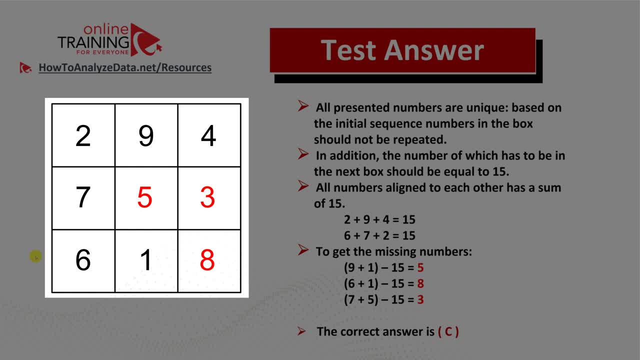 numbers are unique. You can just determine the missing numbers by finding the numbers that are not presented yet on the square. Second pattern that we see here is that all the numbers horizontally and vertically add up to the same number, And this number is 15.. For example, 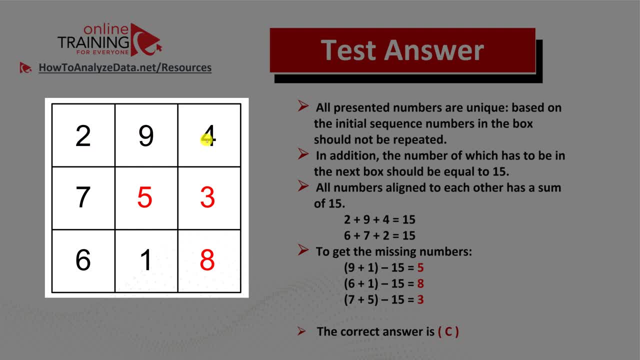 based on the numbers already known, 2 plus 9 plus 4 is 15.. 2 plus 7 plus 6 is 15.. So you can pick the numbers based on this knowledge and find the missing numbers based on uniqueness, and put them. 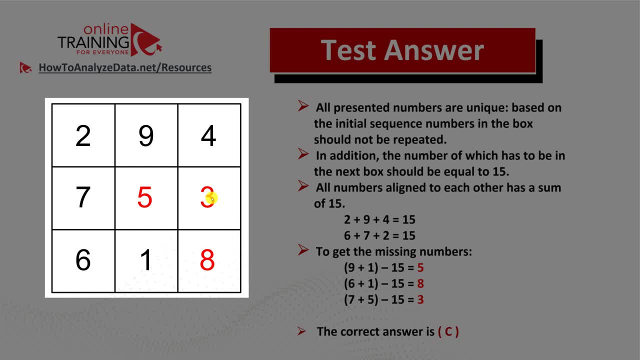 in the right places, Based on the second pattern that we see. Funny thing is you also see that diagonally, numbers also add up to 15.. 2 plus 5 plus 8 is 15.. And then 4 plus 5 plus 6 is also 15.. So the correct. 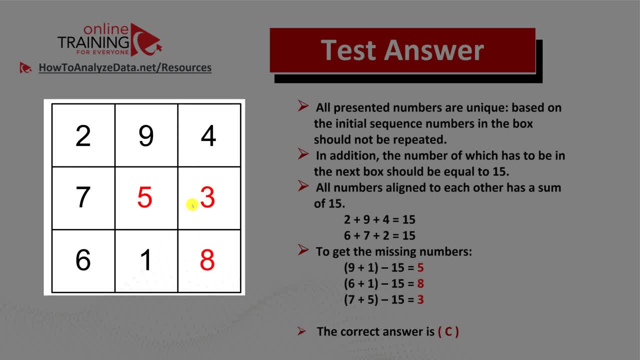 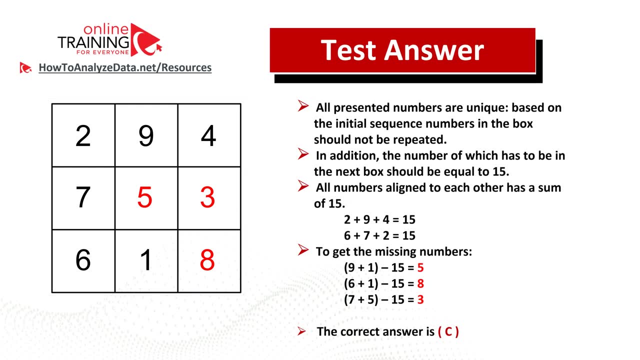 answer here is choice C, And the missing numbers are 5,, 3, and 8.. Hopefully you've nailed this question on your own, Or if you didn't learned how to answer similar questions in the test, But in case you need more questions or practice problems, 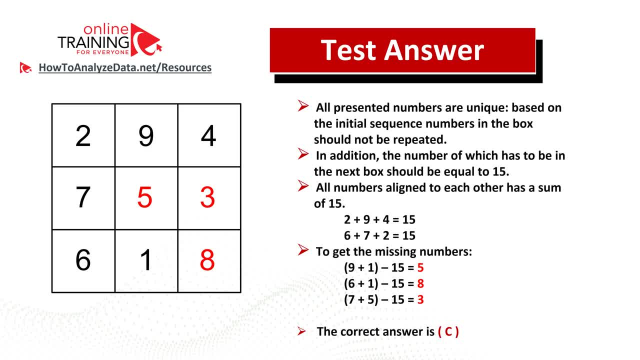 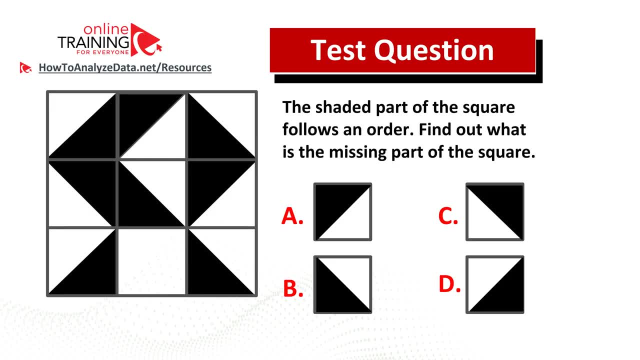 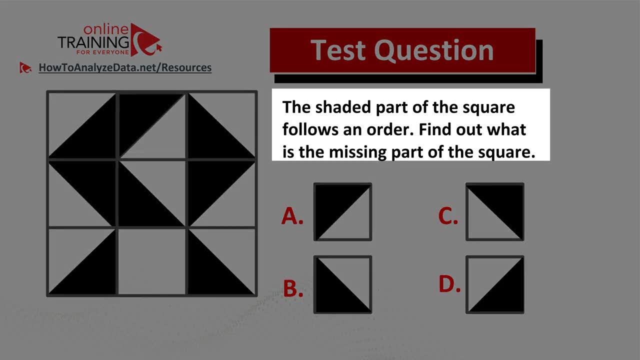 check out my ebook in the description section of this video. The question here is quite tricky, but I would like to show you the solution which, as you will see, is quite simple: The shaded part of the shade. follow the order, Find out. 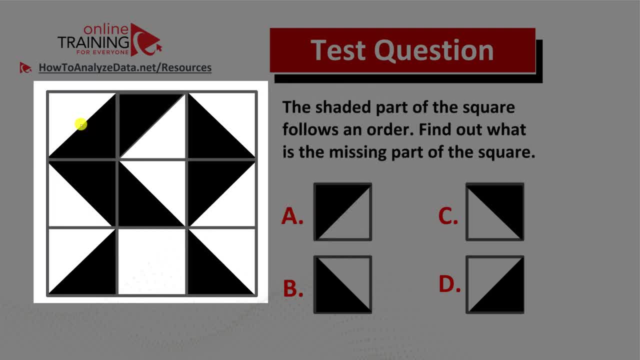 what is the missing part of the square? And you are presented with the 3x3 square And one box inside the square on the lower part in the middle is missing. You need to pick a replacement square out of four possible choices: Choice A, B, C and D. 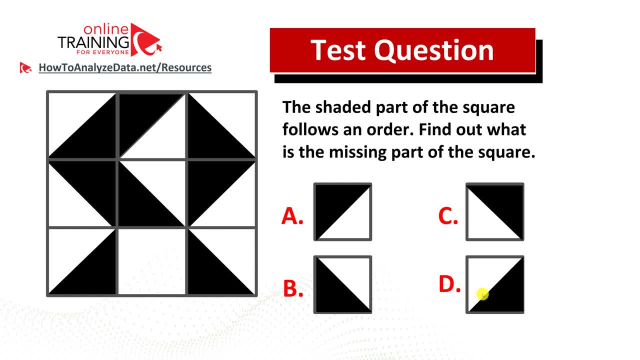 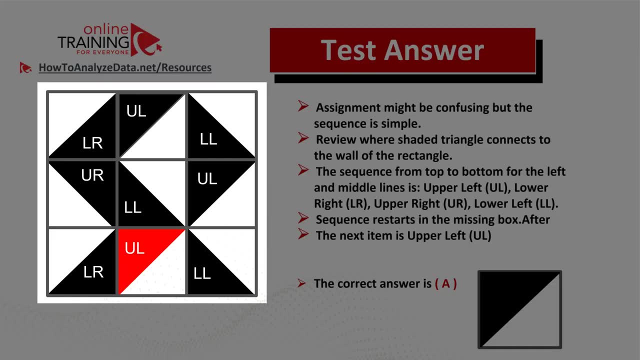 Do you think you know the answer? Now might be a good time to pause the video to see if you can come up with the solution on your own. Do you think you know the answer? Let's continue to see how we can solve this challenge together and get to the correct solution, As usual, to solve these. 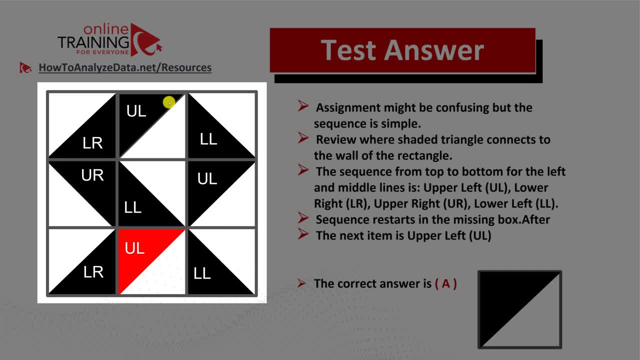 types of questions. you need to look at the sequence, And sequence is determined by where the dark triangle connects to the inside walls of the rectangle. So, for example, if you look at the left and middle line, this is where the sequence is- You see that it starts with upper left. So we 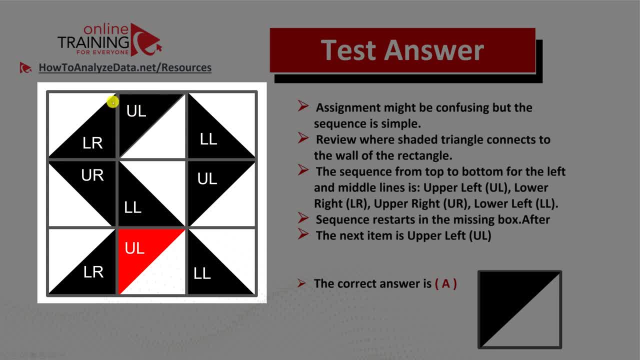 have upper connection and then left connection, Then goes to lower right. So we have lower connection and then right connection, Then goes to upper right And then goes to lower left, And then this is the missing box where we need to find the missing square. 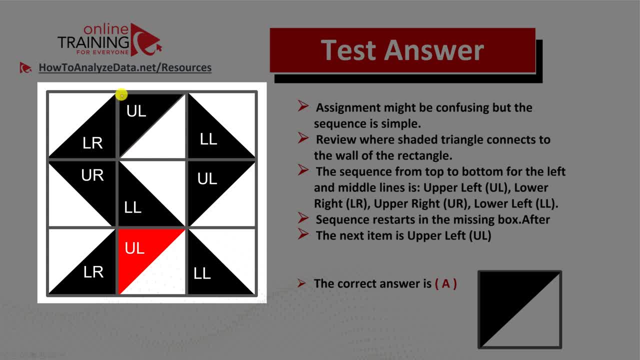 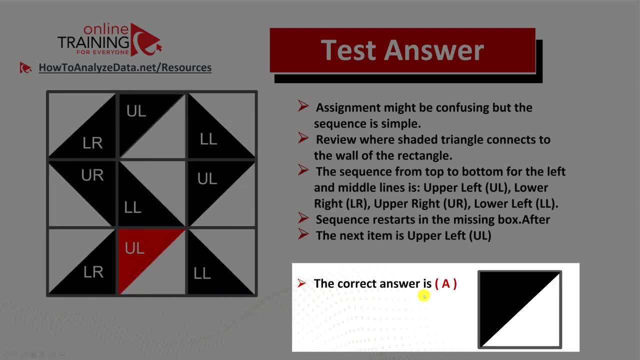 And you see that the pattern here restarts. Upper left was the first item in the sequence, So the next item in the sequence would be upper left again. So the correct choice here is choice A- upper left. Hopefully you've nailed this question. 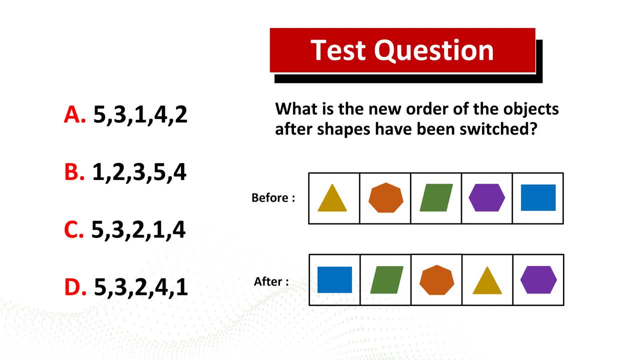 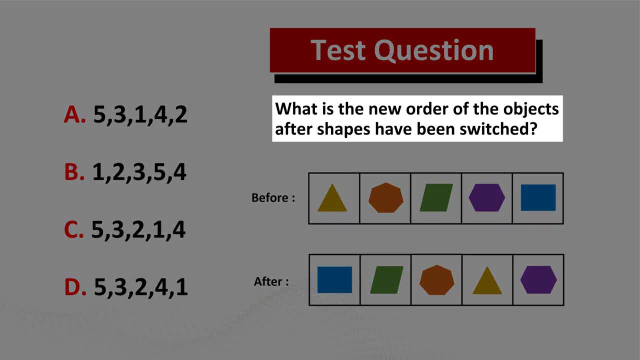 And now here's the question for you to try. Please make sure to post your answer in the comment section of this video and I'll give you my feedback. What is the new order of the objects after shapes have been switched And you have before picture. 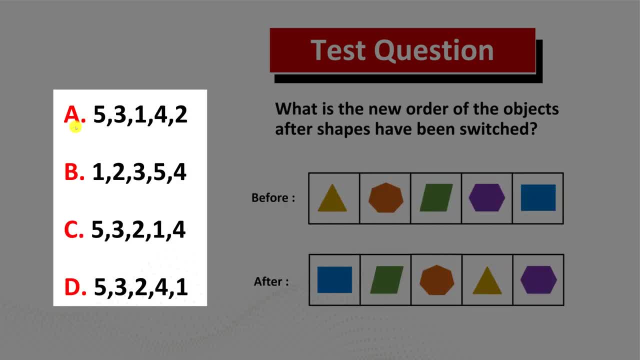 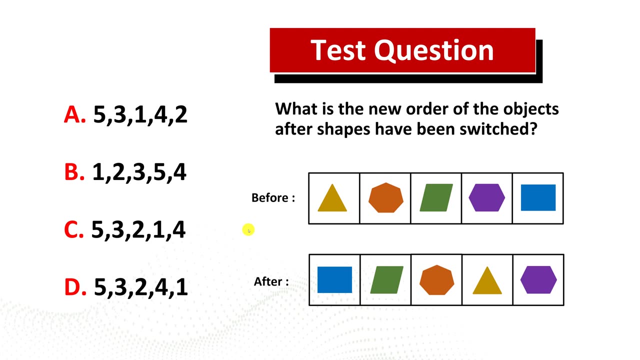 as well as the after picture, as well as four different choices presented. The four different choices reflect new position of the object based on the original position of the object in before picture. Feel free to pause this video and try to solve this challenge And if you came up with the answer, feel free to post it in the comments So I'll give you. 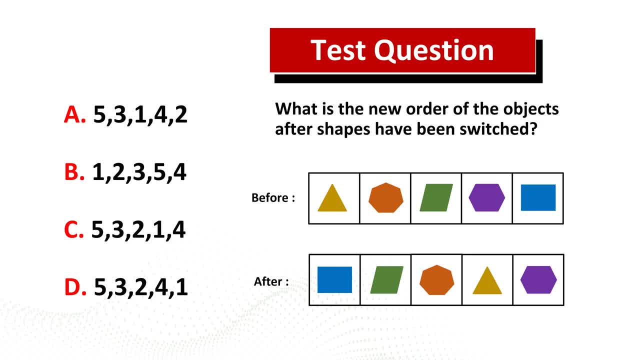 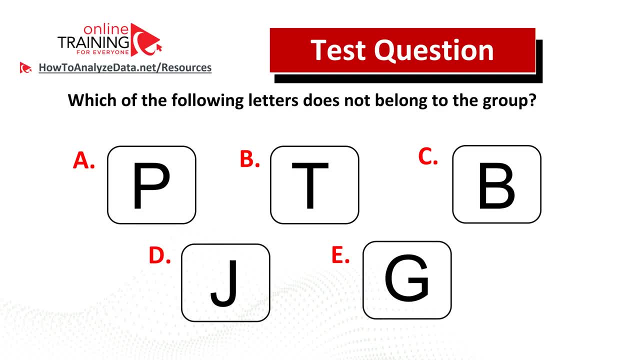 my feedback. Thanks for participating. Some of you might find this question tricky, But regardless of whether you can solve it or not on your own, you will be excited to learn the solution to this real life assessment test question. Which of the following letters does not: 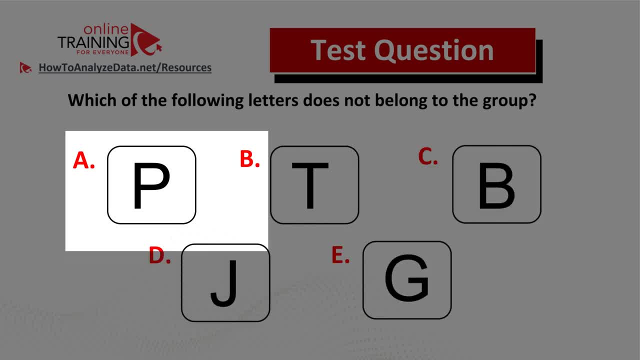 belong to the group And you have five different choices: Choice A- letter P, Choice B- letter T, Choice C- letter B, Choice D- letter J And choice E- letter G. Do you think you know the answer? 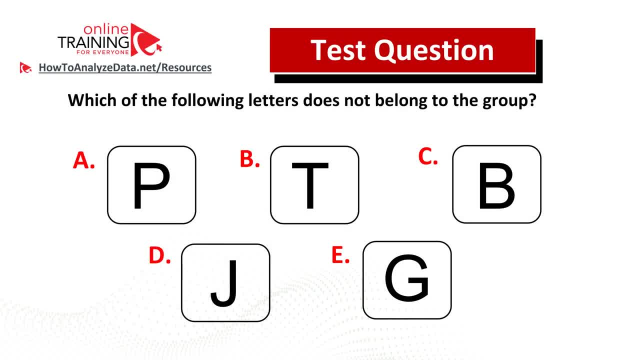 Now might be a good time to pause this video to see if you can come up with the answer on your own. Let's continue to see if we can solve this challenge and get to the solution together. Before we jump to the solution, I would like to give you a clue: Always look for patterns. 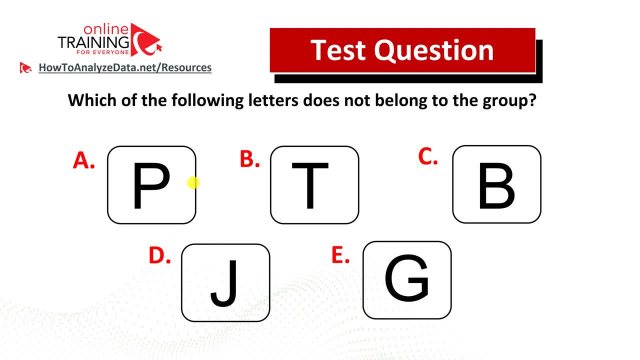 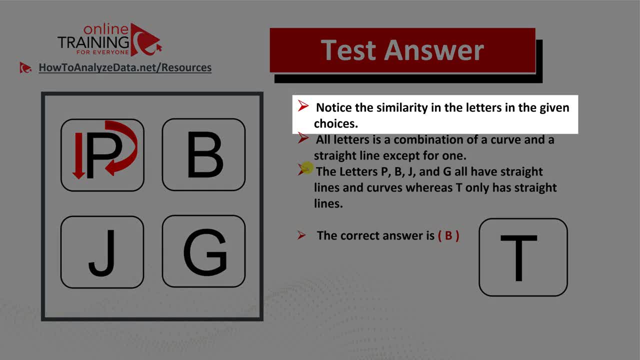 And the pattern here might be sharp edges versus rounded areas for the letters. Now let's go ahead and jump to the solution. When you look at the patterns, you can notice the similarities in the letters for the given choices. All letters are a combination of the. 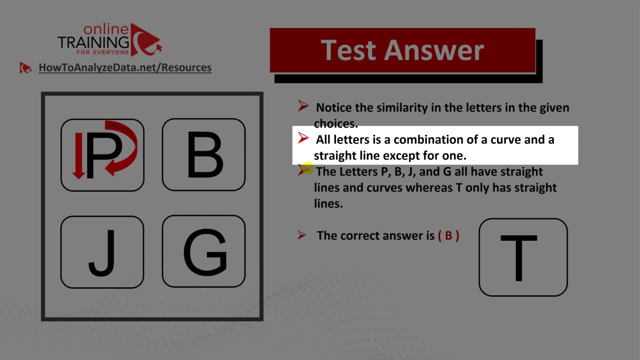 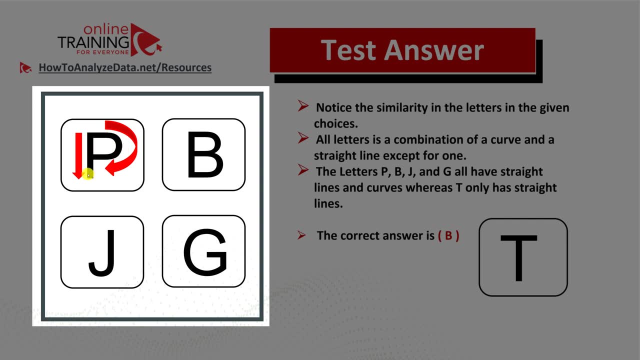 curve as well as straight line. with the exception of one, The letters P, B, J and G presented here, they all have combination of curve as well as straight line. The only letter that does not match this pattern is letter T, So the correct choice here. 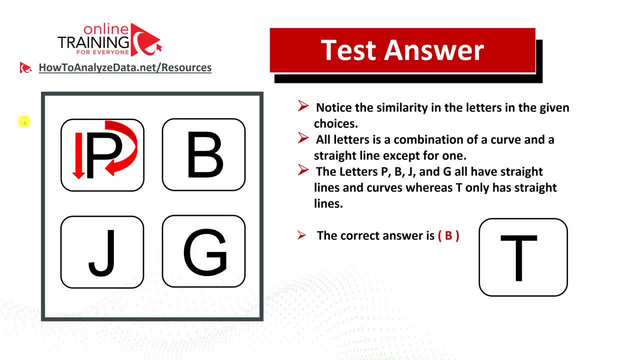 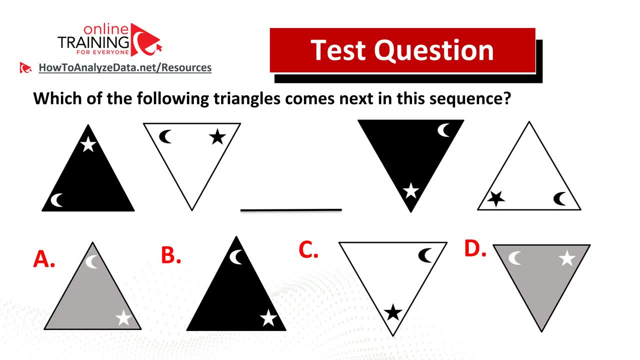 is choice B, letter T. Hopefully you've nailed this question All right. I have a tricky question for you which you might frequently see on the test. The cool thing is that you might be able to solve it. Or, in case you don't, I would love to show you the solution. 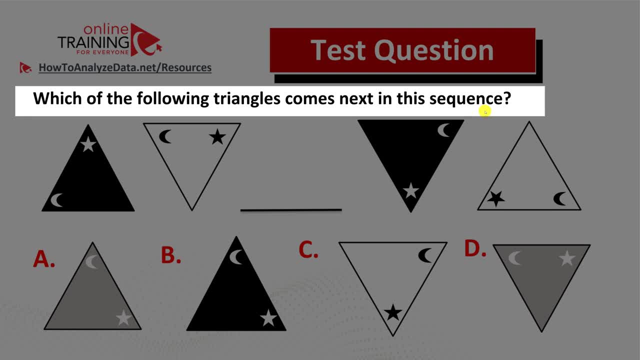 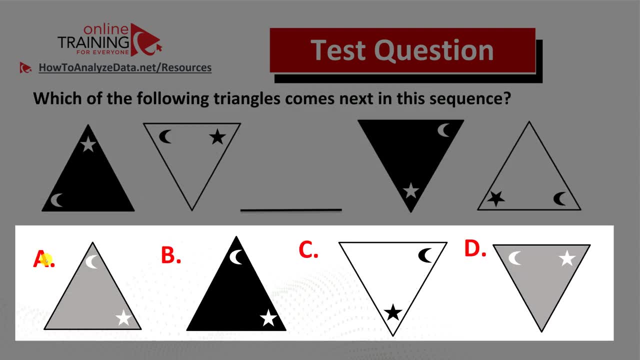 Which of the following triangles comes next in the sequence? You have a sequence of five triangles And one triangle in the middle is missing, And you have four different choices to pick the right triangle. Choices A and B, represented by gray and black triangles pointing toward the top. 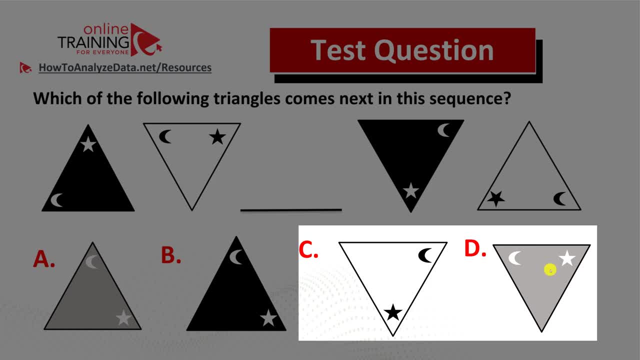 And choices C and D, represented by white and gray triangles pointing to the bottom. Do you think you know the answer? Now might be the right time to pick the right triangle. Now might be the right time to pick the right triangle. Now might be the right time to pick the right triangle. 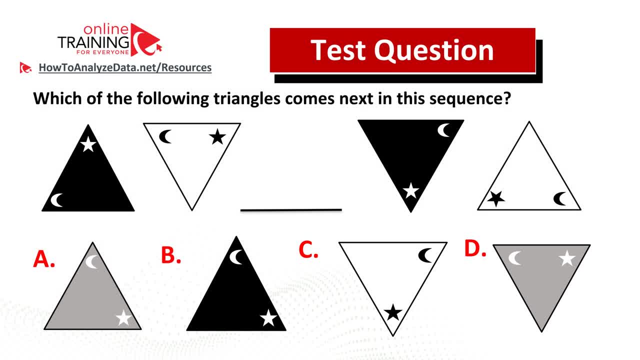 Pause this video to see if you can come up with the answer on your own. Do you think you came up with the answer? Let's continue to see how we can solve this challenge together. Before revealing the solution to you, I would like to point. 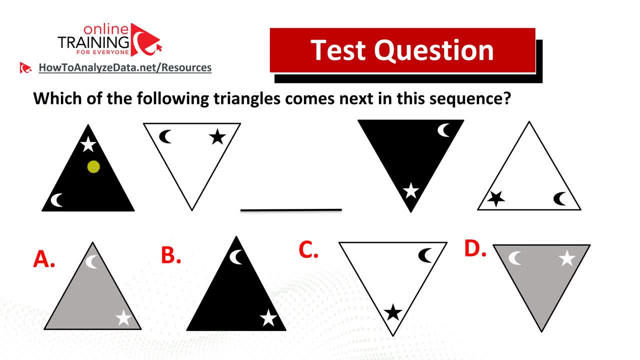 at two patterns that we see in this problem. The first is the pattern of colors. You have black triangle, white triangle and then missing triangle, Then black triangle and white triangle. So something might be different from black and white. So something might be different from black and white. 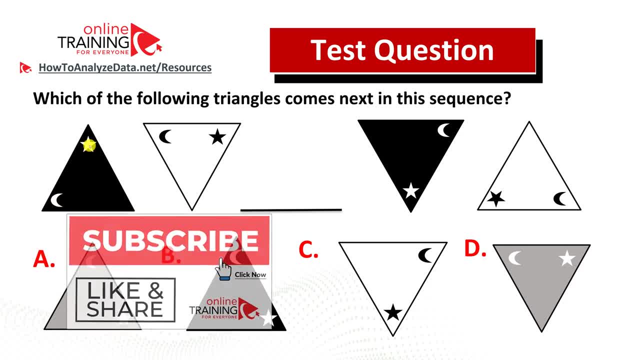 Potentially here You also have a pattern of moon and star And moon and star. they move inside the triangle. So you see moon and star in the leftmost triangle, Then you see moon and star on the top, Then you see moon on the top and star at the bottom. 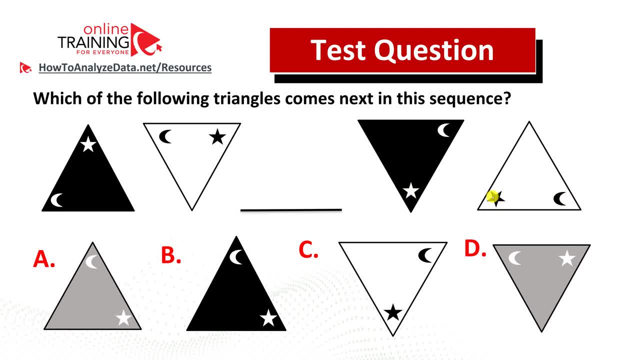 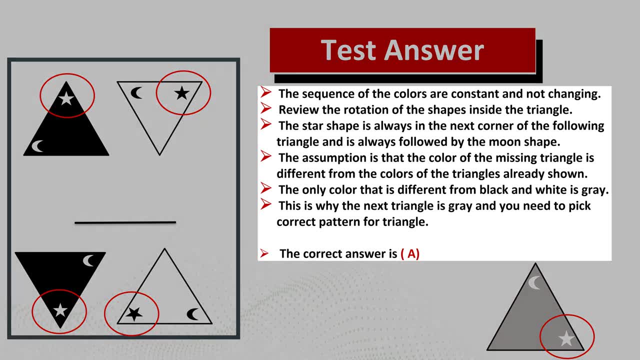 And then you see both of them: moon and the star at the bottom of the triangle. So now let's jump to the solution. We have already looked at the pattern of the colors and the sequence of colors is constant And is not changing. 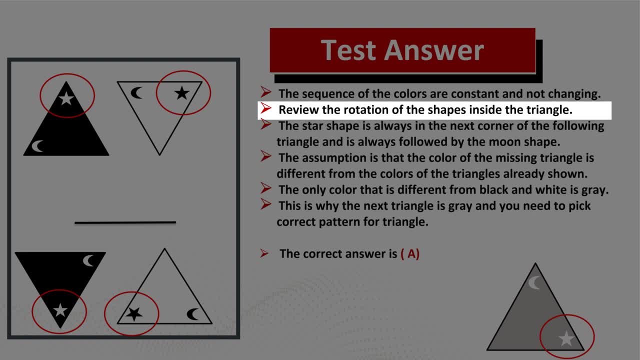 And we also reviewed the rotation of the shapes inside the triangle. The star shape is always in the next corner of the following triangle And is always followed by the moon shape. The assumption here is that the color of the missing triangle is different from the colors of triangles already shown. 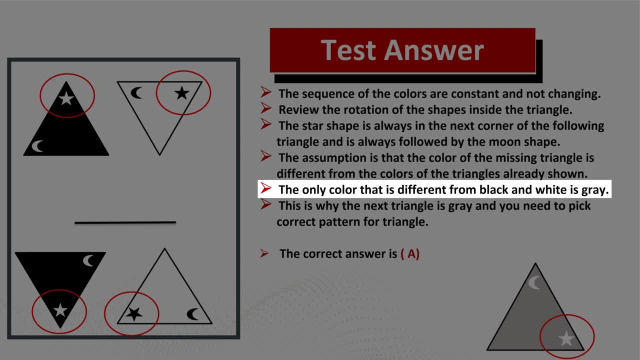 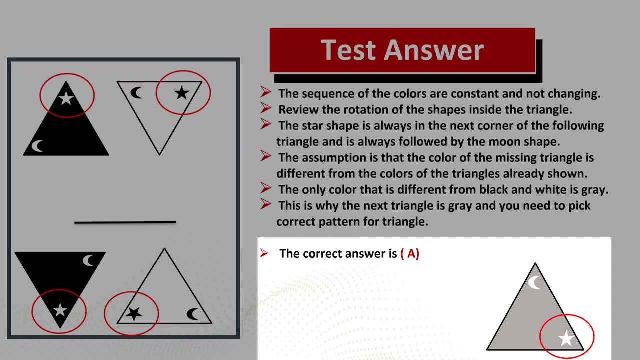 And the only color that is different from black and white is gray. This is why the next triangle is gray, And you would need to pick correct pattern for the triangle. So the correct choice here Is choice A. There are two gray triangles here. 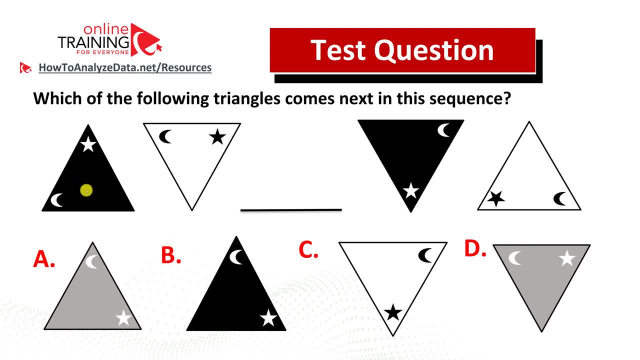 Choice A and choice D. But there is also a third pattern Pattern that I did not mention Because it will make things very obvious, And this is the pattern of pointing. You see that the first triangle is pointing upward, The second triangle points down. 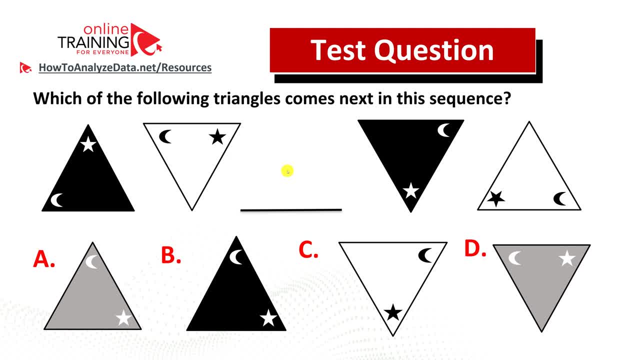 So the next triangle in the pattern will be pointing up as well, And the only gray triangle that points up is choice A. Hopefully you've nailed this question And now know how to see the patterns And solve the problem And solve these types of challenges on the test. 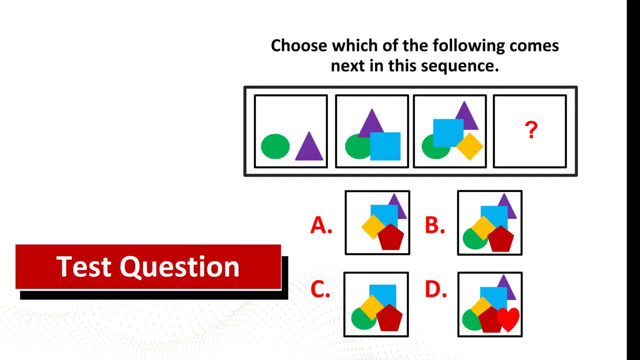 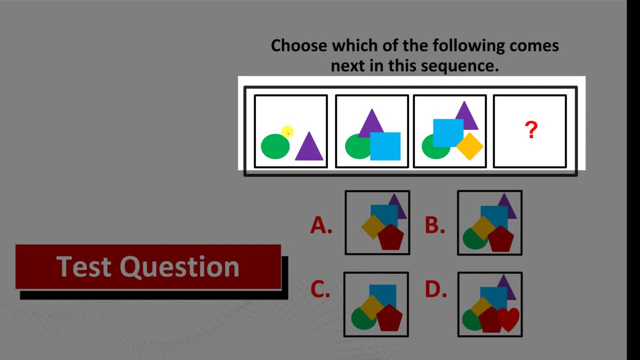 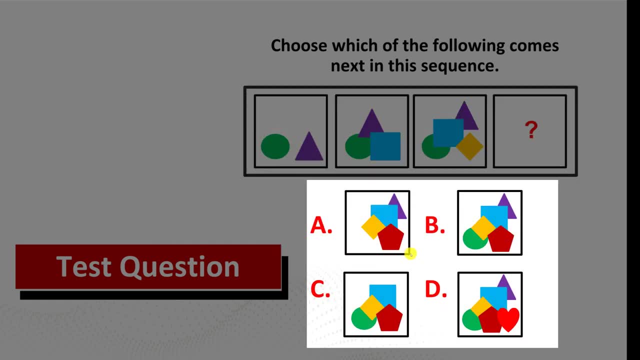 And now here's the question for you to try. Please choose which of the following comes next in the sequence. You are presented with the sequence of objects, And the fourth object in the sequence is missing, And you have four different choices presented here. 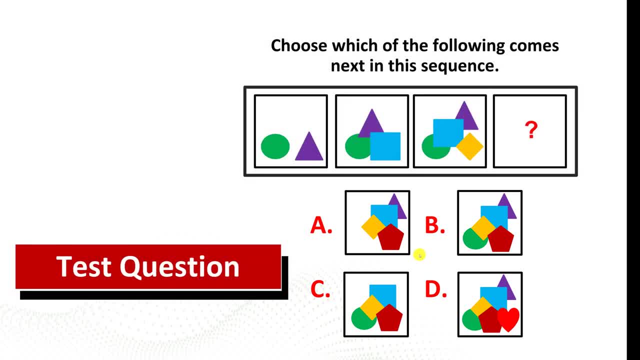 And you need to select one out of four choices. Feel free to pause this video and try to solve this challenge. Did you come up with the answer? Feel free to post it in the comments. Feel free to post it in the comments section of this video. 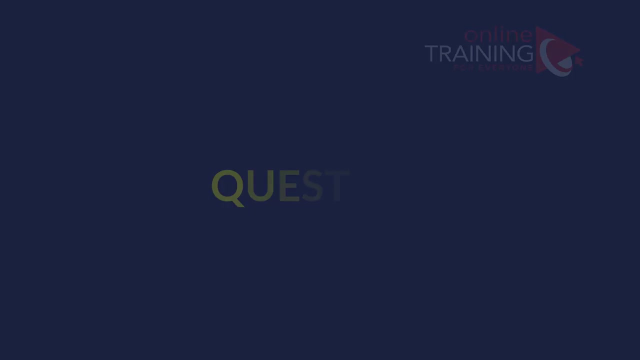 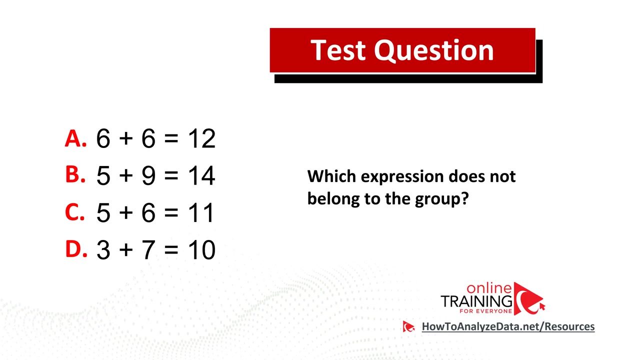 And I'll give you my feedback. Thanks for participating. Let's see if we can solve this challenge together. Here is the very interesting and at the same time tricky question you might frequently see on the test Which expression does not belong to the group. 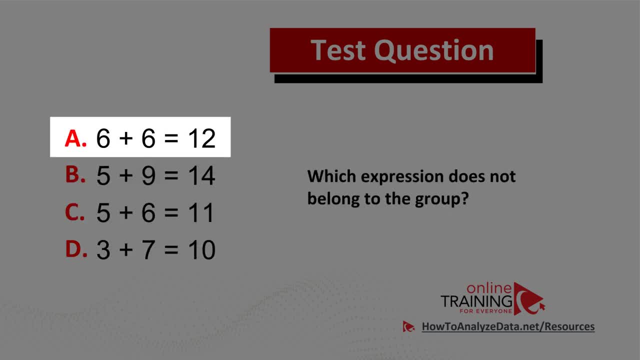 And you have four different choices: Choice A: 6 plus 6 equals 12.. Choice B: 5 plus 9 equals 14.. Choice C: 5 plus 6 equals 11.. And Choice D: 3 plus 7 equals 10.. 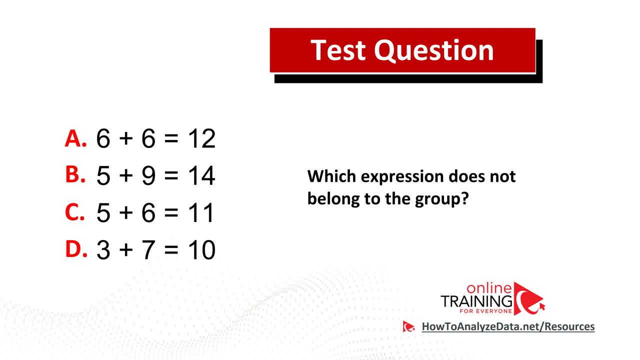 Do you think you know the answer? Now might be the right time to pause this video to see if you can come up with the answer on your own. Give yourself 10 or 20 seconds and see if you can come up with the solution. 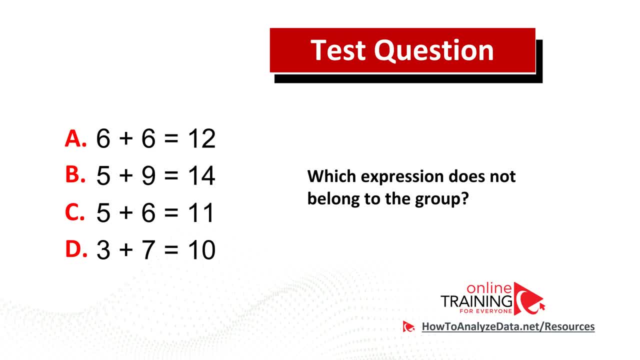 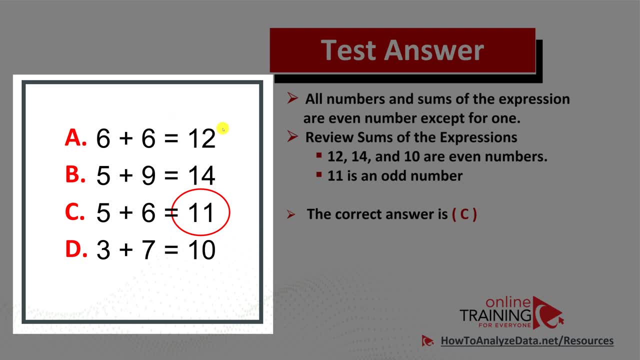 Did you come up with the answer. Let's continue to see if we can solve this challenge together. Let me show you two ways you can solve this challenge. First, let's look on the right side of the expression. You see that the twelfth and the twelfth are the same. 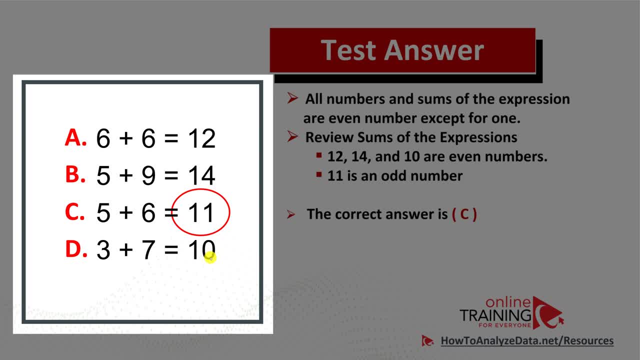 12,, 14, and 10 are all even numbers And 11 is the odd number. So that should give you some clues. If you look on the left side of the expression, you see that 6 plus 6 is the combination of even numbers.